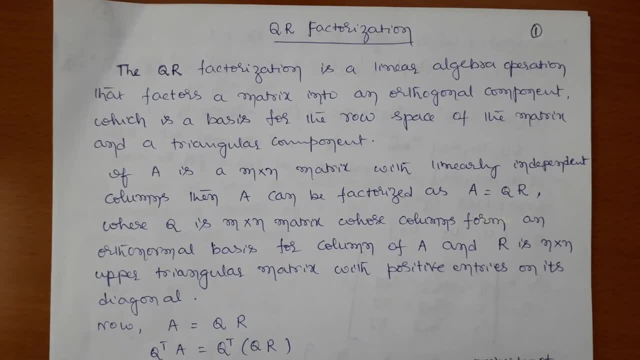 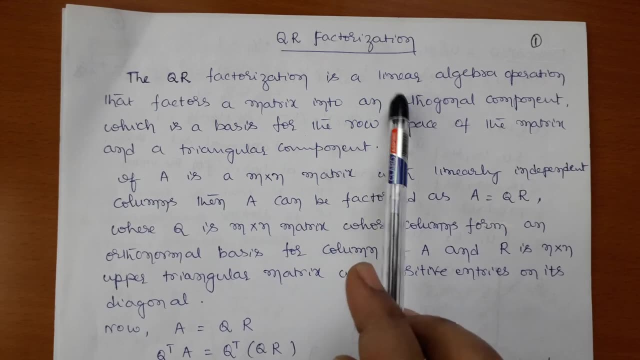 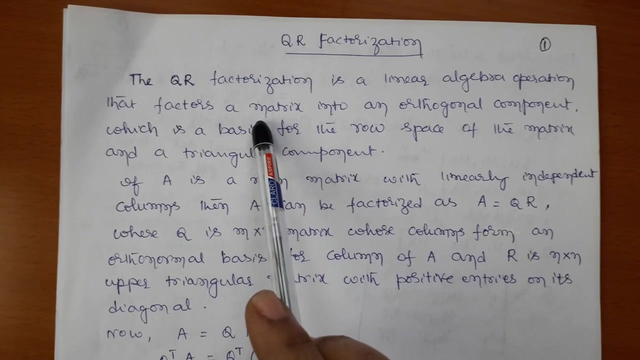 previous videos for Gram-Schemit process, The continuation of Gram-Schemit process, we get QR factorization. The QR factorization is a linear algebra operation. It is a linear algebra operation That factors, this is factors a matrix into an orthogonal component, which is a basis for the 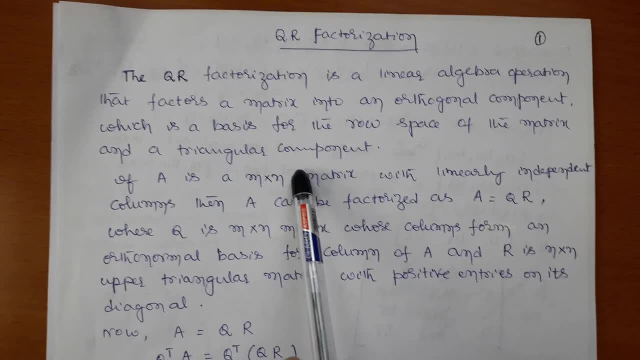 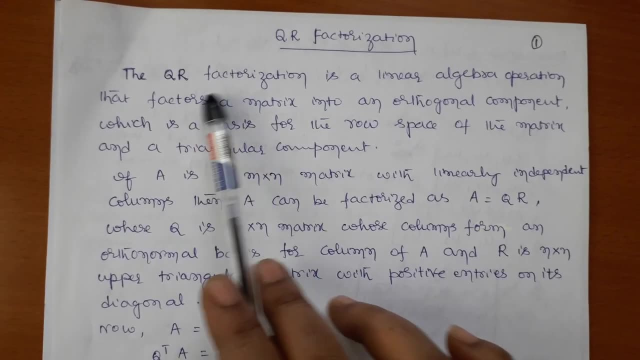 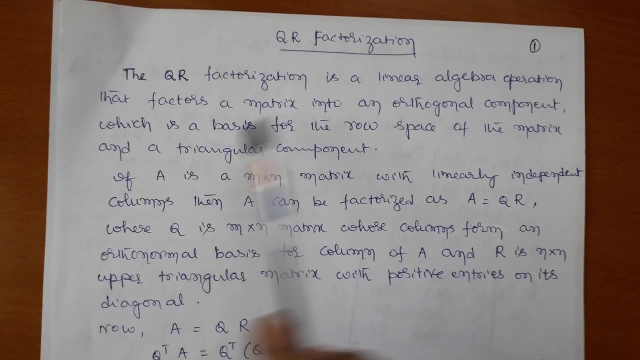 row space of the matrix and a triangular component. They divided into the given matrix into two matrix factor into two Q, into R. Q is nothing but is a matrix into that matrix having a orthogonal component. This is a which is a basis for the row space of the matrix and 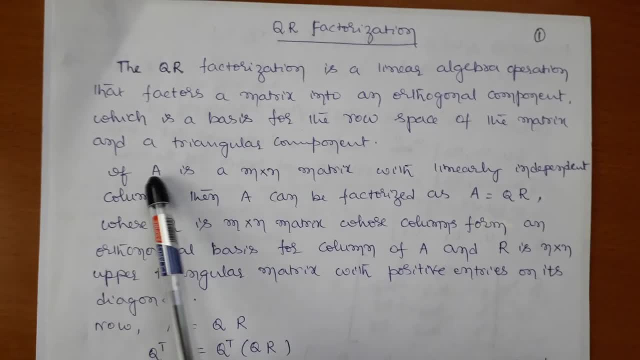 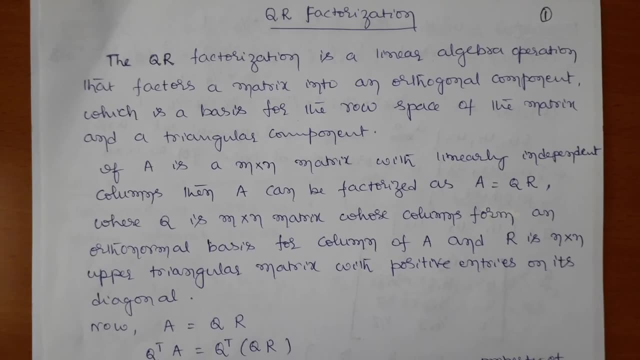 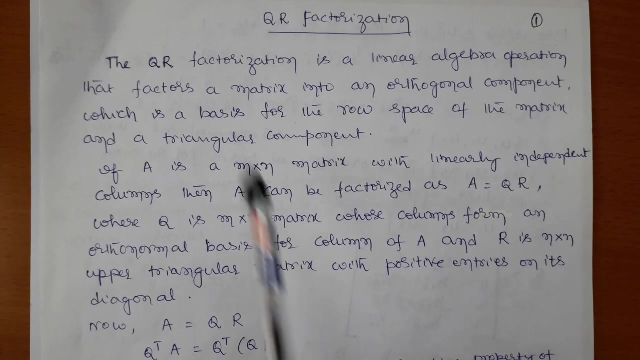 also another matrix, AH, R is a rectangular components, They totally the given matrix, divided factors, factorized into two. one is Q and R. Q is having orthogonal, ortho normal basis for the matrix, they having a column, and R is having a is a rectangular, a matrix they have not a. 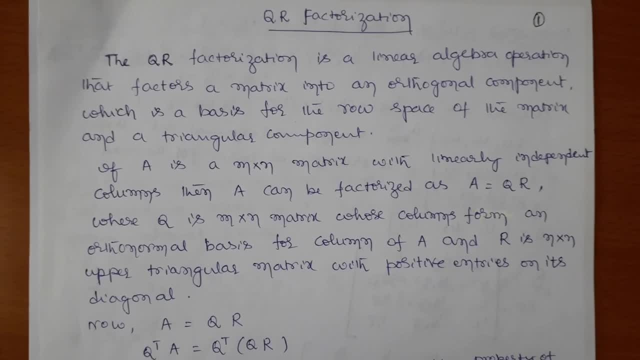 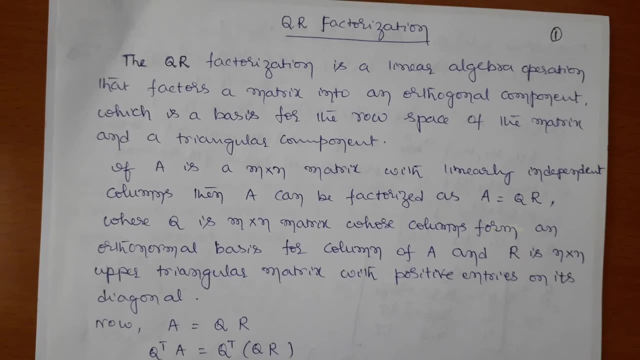 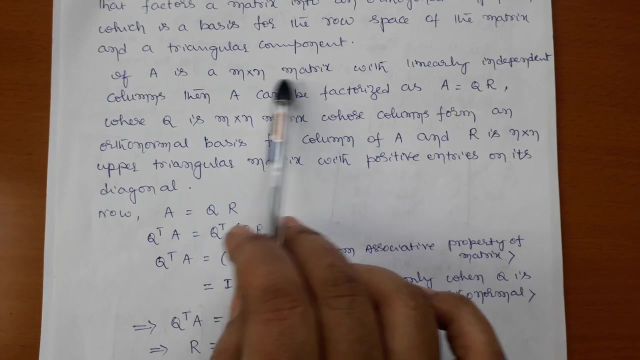 rectangular component Means they having a rectangle is a. R is a rectangular matrix. Therefore total is divided into factors in the rectangular components. Then R is a triangular matrix. into how many matrix? 2 you want r? yeah, if if a, if a is an m cross n matrix, they given a matrix. 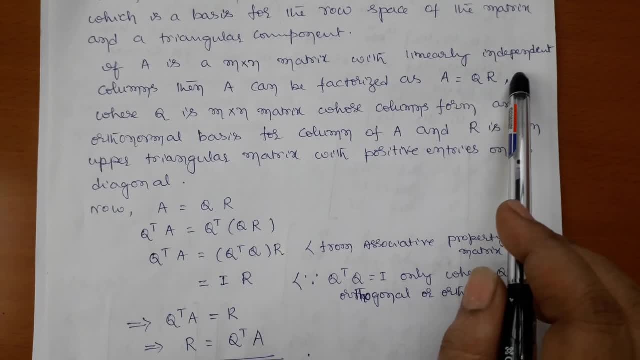 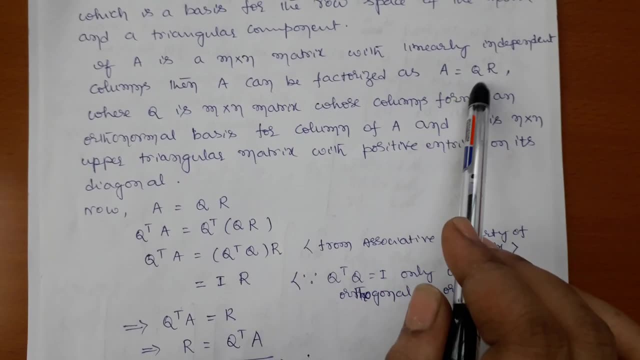 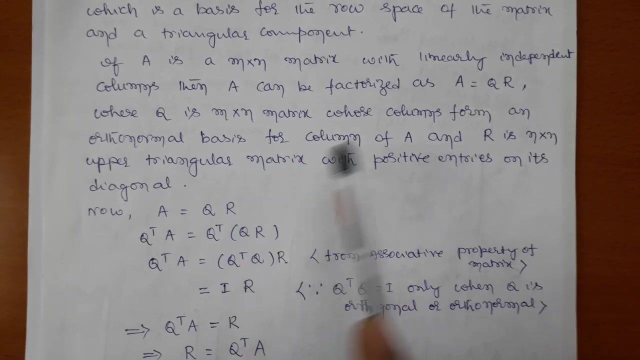 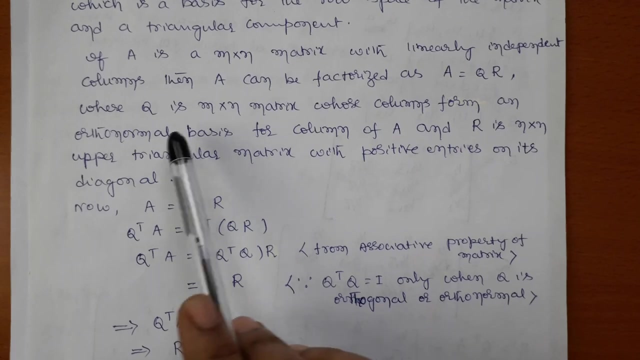 they having m rows with n columns, with linearly independent columns- they talking about columns are linearly independent- then a can be factorized, as a is equal to q, into r, where q is a. m cross n matrix whose columns form an orthonormal basis of the columns of a, you form a columns of q. 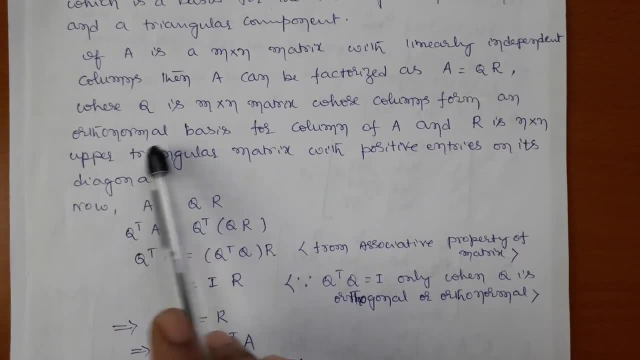 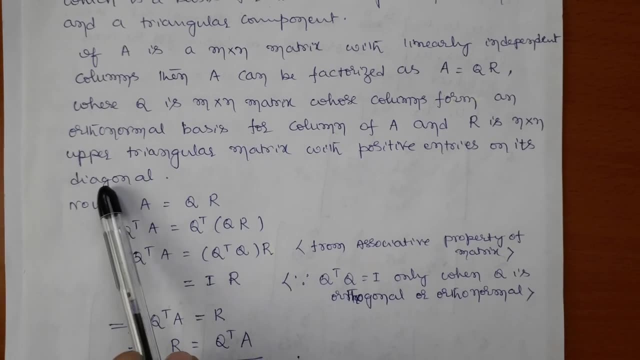 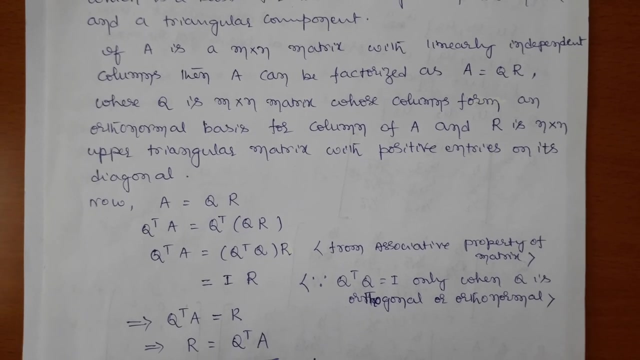 is m cross n matrix whose columns are form from orthonormal form. an orthonormal basis for the columns of the matrix a and r is n cross n upper triangular matrix with positive entries on its diagonal. in the diagonal always, you are expecting, the entry must be positive. yeah, before moving to, 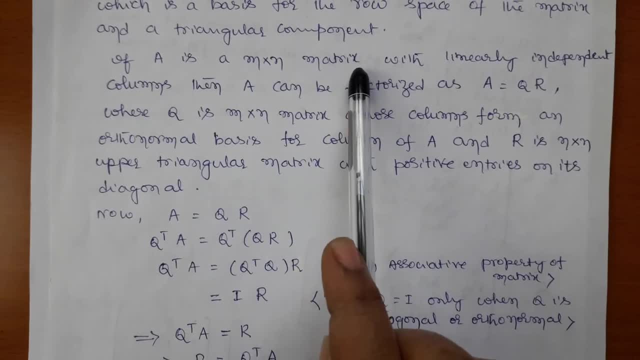 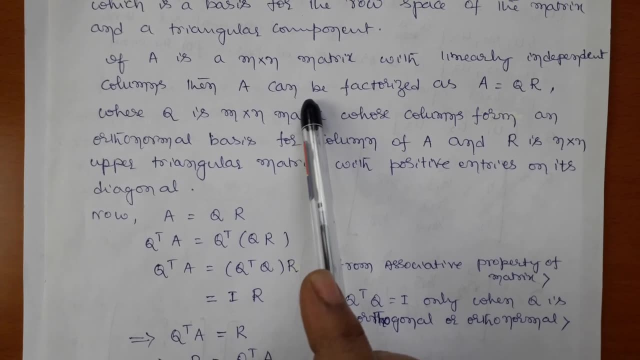 the next slide. next step. please try to understand. if a is a m cross n matrix, okay, with the matrix having. what type of matrix you are expecting with linearly independent columns? then a: yeah, you have a matrix. you can't convert directly that. my every matrix is q into r, each of the column of the. 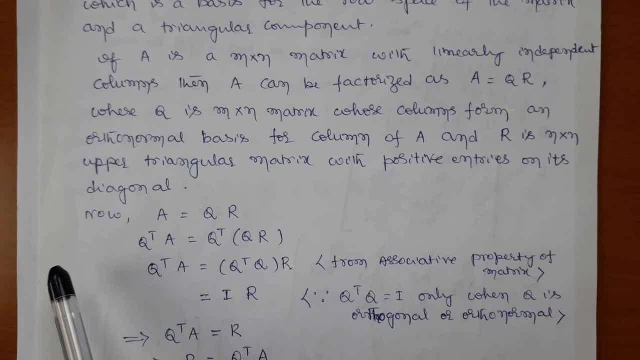 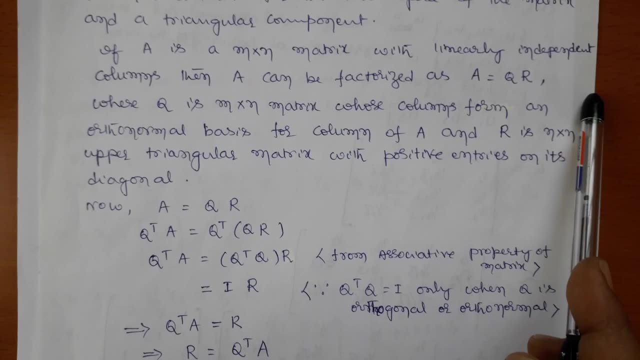 matrix is, must be a linearly independent. you already know that. what's the definition of linearly independent, then only is possible: i have to factorize a as q into r, where q is a m cross n matrix whose columns form a m cross n matrix whose columns form an orthonormal basis of the columns. 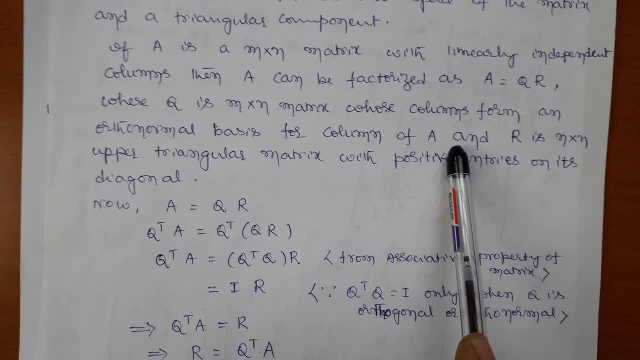 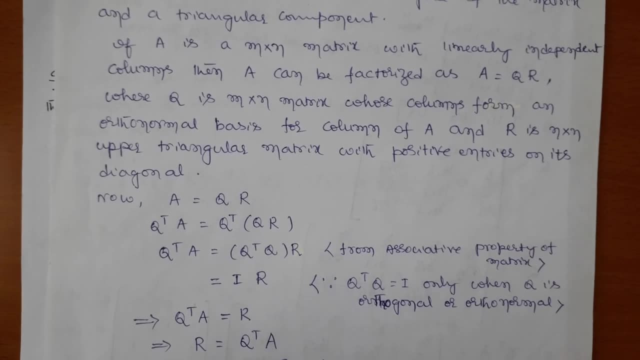 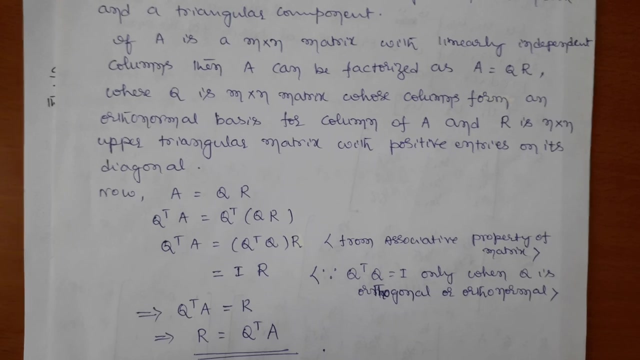 form. an orthonormal basis for the columns of the matrix a and r is n cross n upper triangular matrix with positive entries on its diagonal. only worried about positive entries in our diagonal. but other than diagonal value may be a negative, but keep in mind that r is a upper triangular matrix. 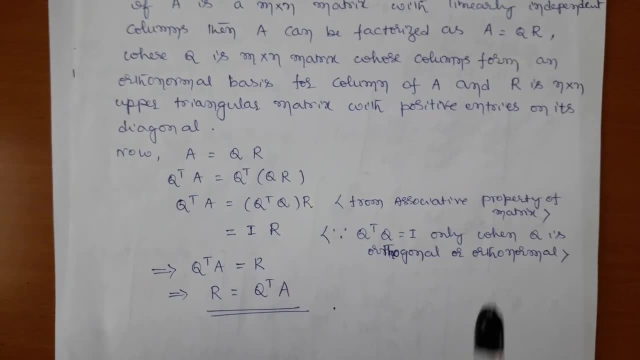 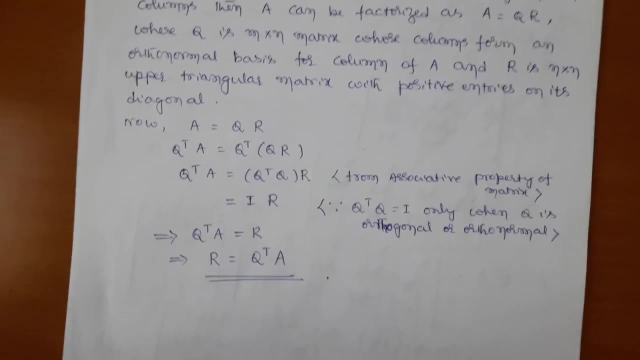 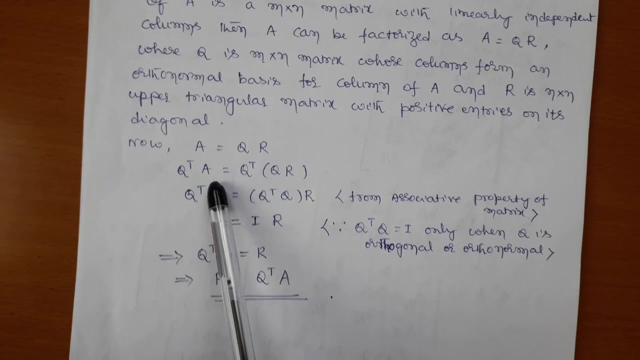 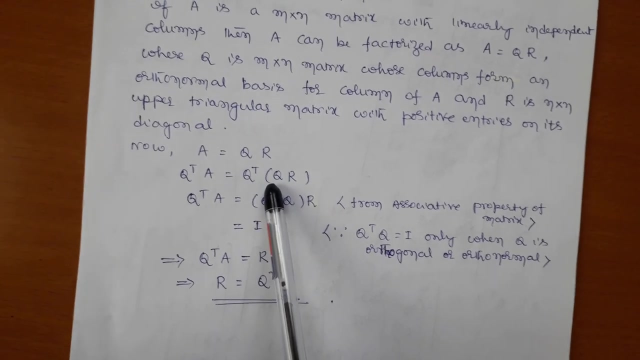 now a equals what we decided. a can be written as what actually. a is nothing but q into r. a is nothing but what q into r. okay, a is q into r. then i'm going to take q transpose on both sides. q transpose into a is equal to q transpose of q into r. q is a matrix, is a matrix form for. 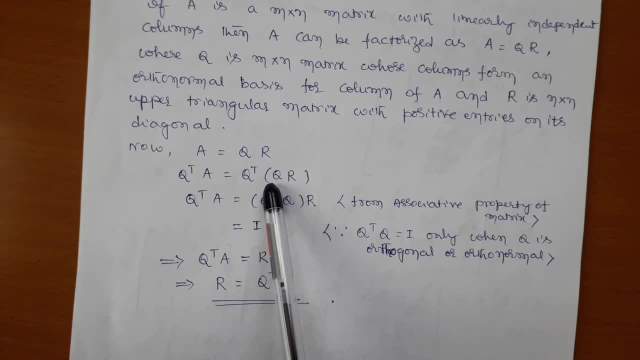 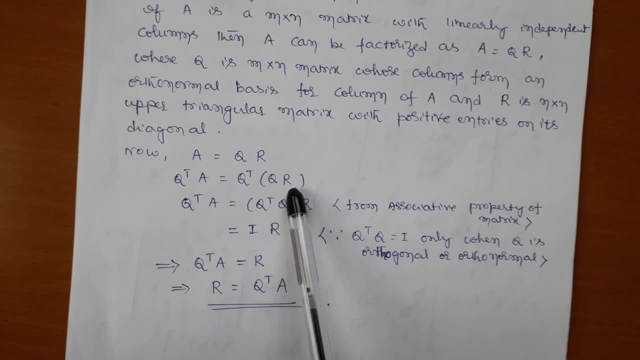 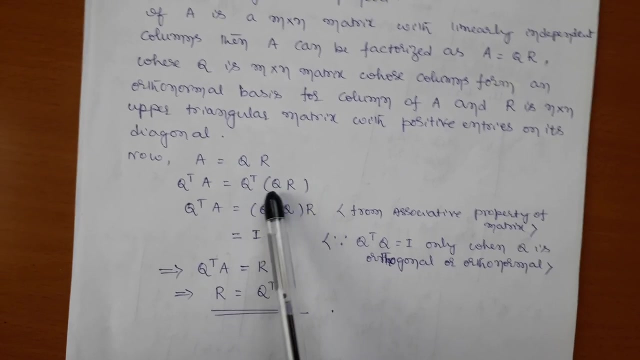 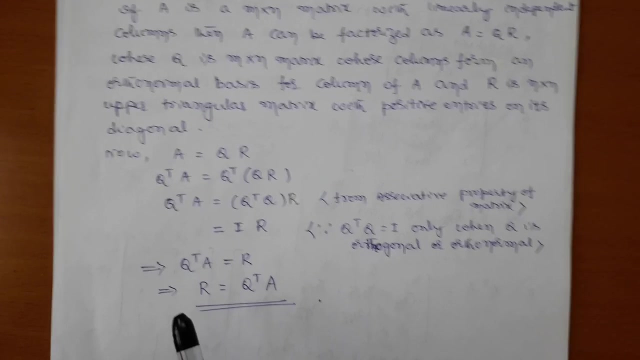 arthur, orthonormal basis for the vector column, vectors of the, the form from the columns of a and r, is a upper triangular matrix with diagonal entries or positive entries, then this is a firm associative property of matrix. either i to group these two or groups these two does not matter, because a into bc is nothing but a, b into c, that associative property. 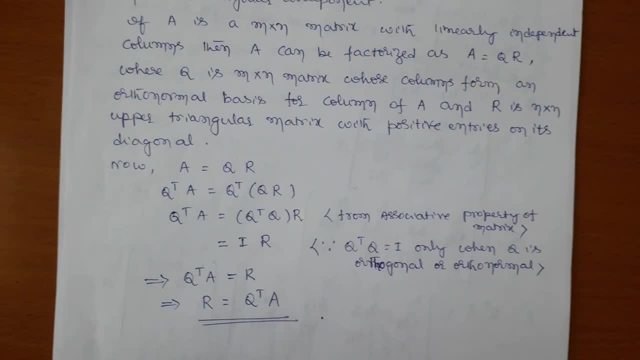 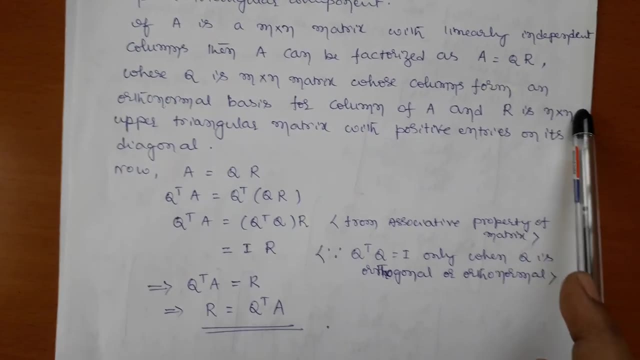 holds could, under the multiplication therefore, group these two. i'll write you this is i, because a is what actually a is formed. a is a m, cross and matrix whose columns form an Night. Under Greek Mathlusion, a n means a column becomes an orthonormal basis for the columns of a. each column is an orthonormal basis of a. each soundfer, Como Museum, Mu base word. 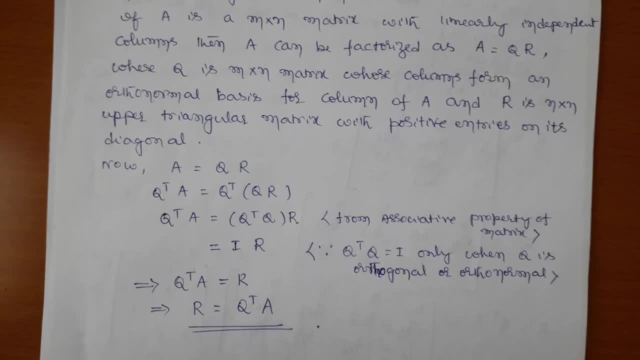 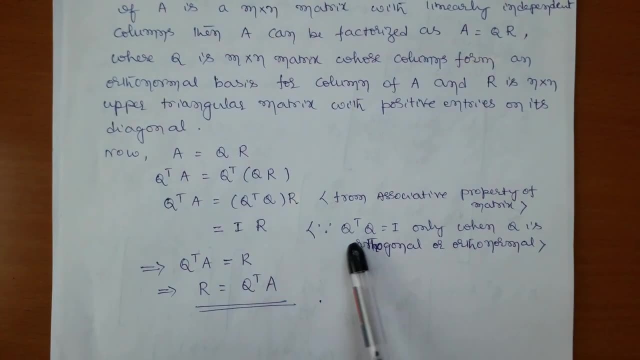 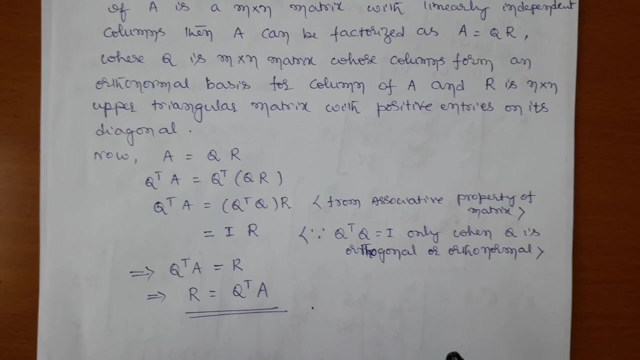 column is orthonormal basis. This orthonormal basis means it must be an orthogonal. Whenever matrix is orthogonal from the basic concept of matrix, the Q transpose into Q is equal to identity matrix. only when Q is an orthogonal or orthonormal, because orthonormal is an orthogonal. 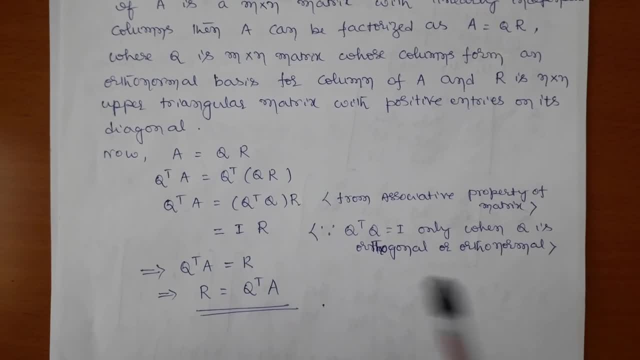 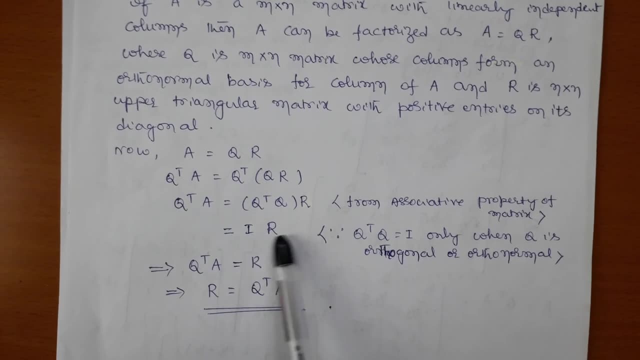 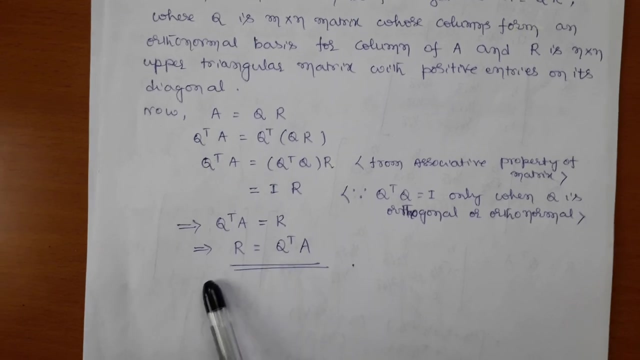 but orthogonal need not be an orthonormal. you already known that? Yeah, now here is orthogonal matrix. therefore, what is Q? transpose into Q is nothing but I, I into R. identity matrix into R itself is R. Therefore, Q transpose into A is equal to R. then what we get R, R is how we get. 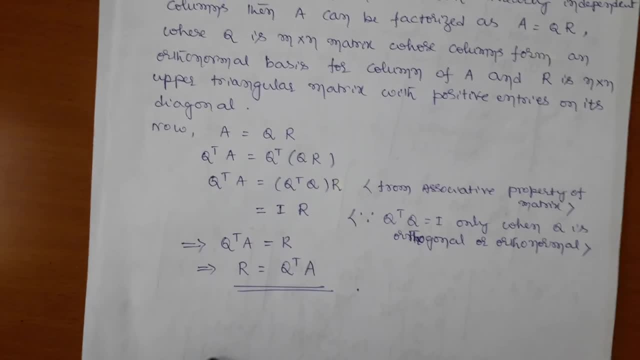 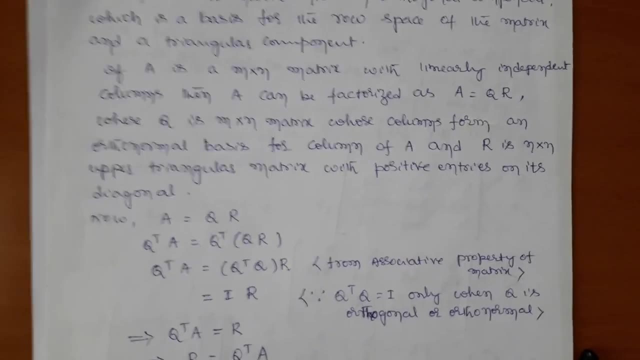 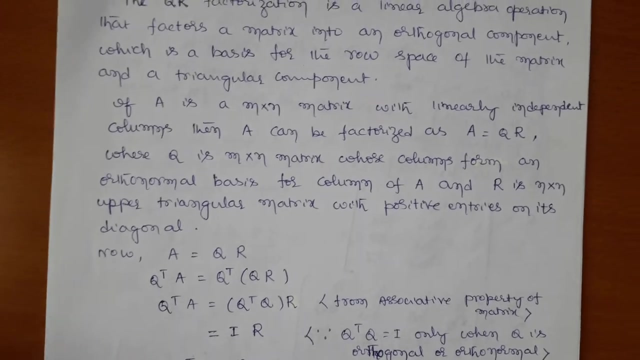 R, Q transpose into A. The entire story of this QR factorization is: if we want to apply QR factorization method, one point we have to observe: In the matrix, each and every columns of the matrix are given. matrix are nothing but linearly independent. Once it is linearly independent, 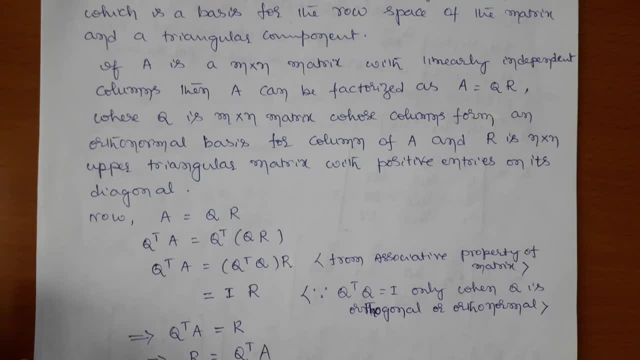 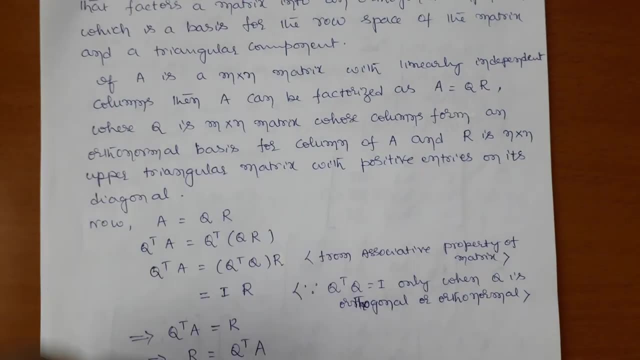 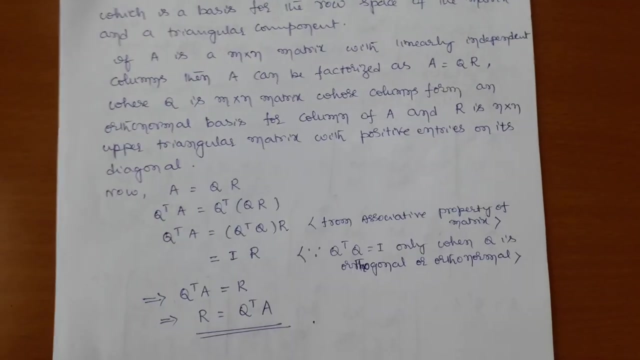 the next. you find out orthonormal basis for the given matrix of A. You take it each column of the vector. then you use Gram schematic process to find out orthogonal set. from that we get orthonormal set. Then each vector you write it in the column of Q. Write it in the column of Q is nothing but. 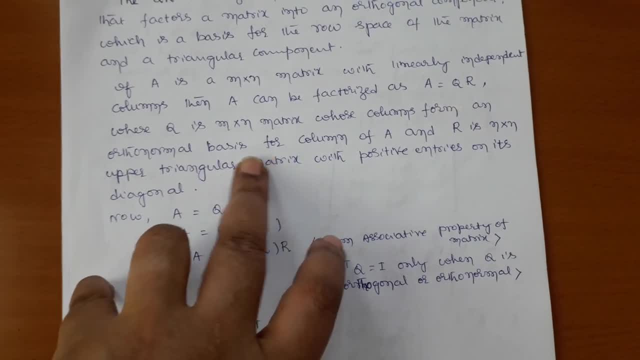 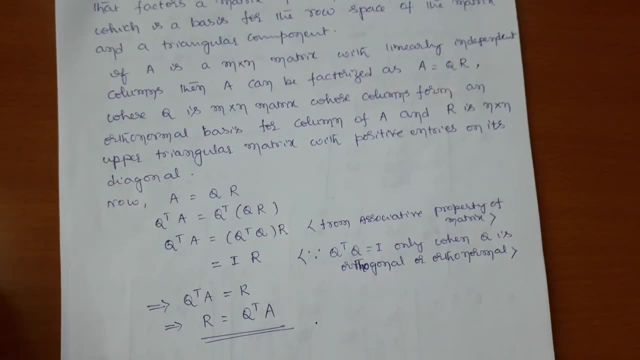 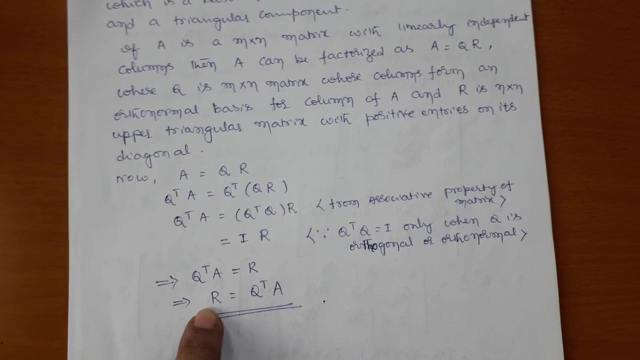 each column of Q is nothing but orthonormal basis for the columns of A. Yeah, after that, how Then we get Q? How to find out R? We are using a formula, for R is what Q transpose into A, Then we get R. Once we get R, for your cross, check what we did. Q and R is correct or not. we get immediately. 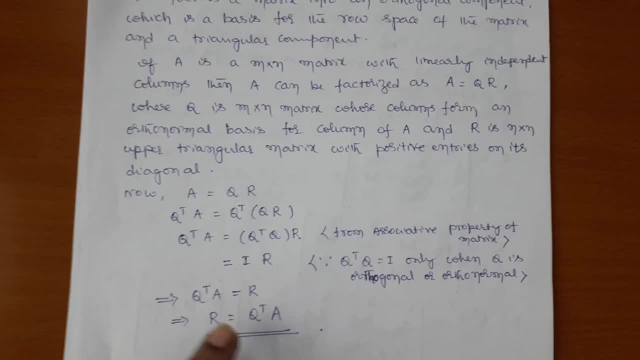 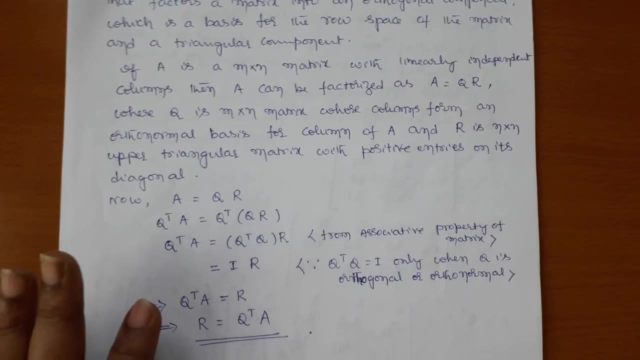 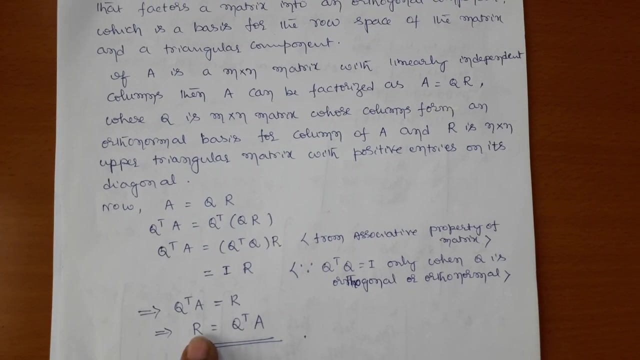 we have a, confidently say that I get a, full marks or not, You multiplied with what we get R, with, along with Q, Yeah, once you get A, then we say that what you factorize A into Q, into R is correct, otherwise not correct. So finding R, keep in mind R is upper triangular matrix, but diagonal point is must be positive. 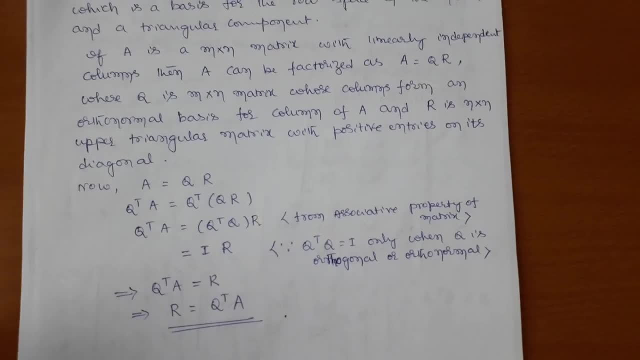 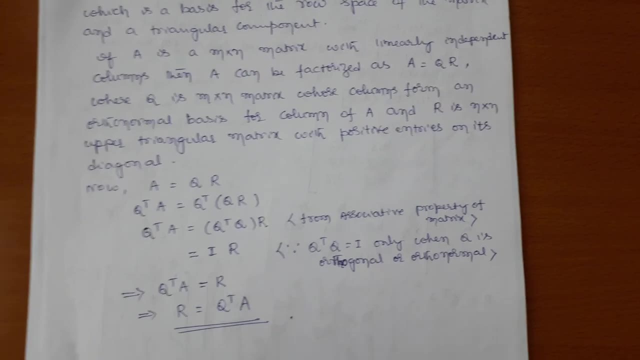 You have to take care for that. Suppose R is we get a upper triangular matrix but any one of the value in the principal diagonal value is whatever that negative value is not a positive, then you have to recheck. maybe you have done some where mistake. You suppose you satisfy these two. 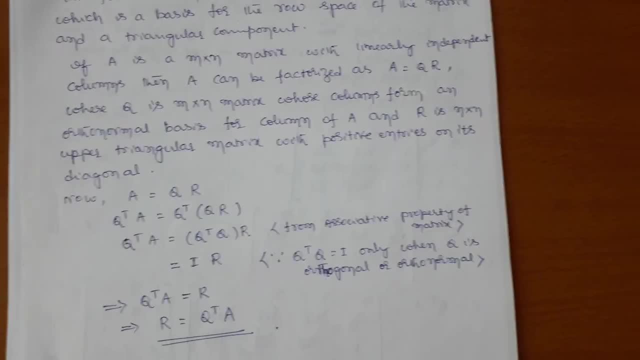 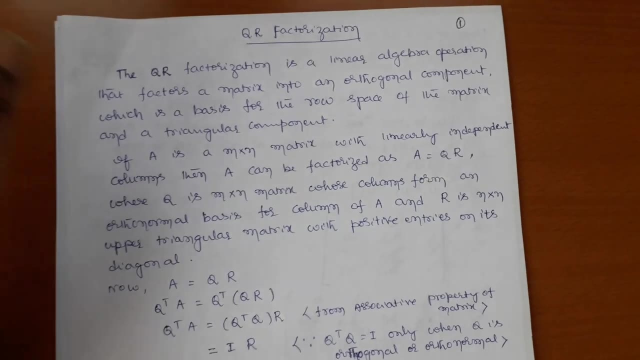 condition. and then you multiply Q into R is equal to get A. Yeah, before moving to the next step, what are the steps I have to follow for to factorize the given matrix into q, into r? first you observe the given matrix a in each of. 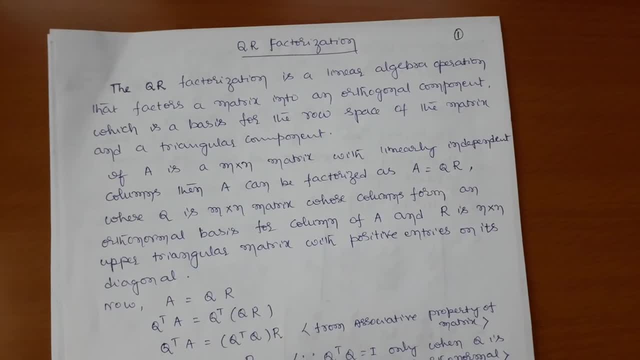 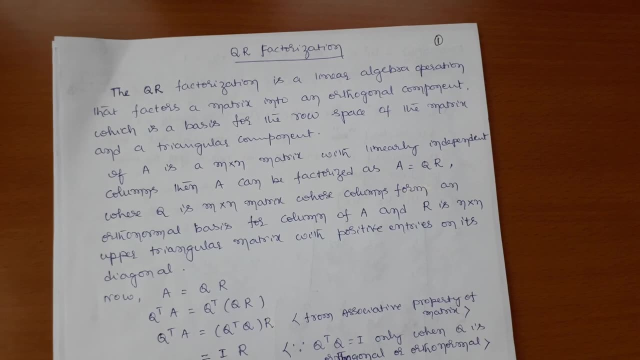 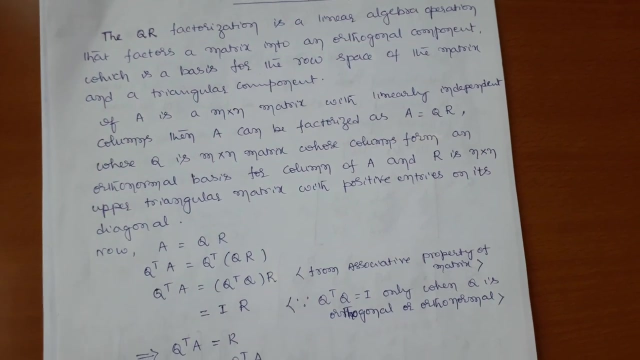 the column of the matrix is nothing but linearly independent. you pick the column for a of the given matrix. that is nothing but vectors. say v1, v2, etc. vn apply grams commuted method to process to find out orthogonal set. from that we get orthonormal basis set and also corresponding orthonormal basis. 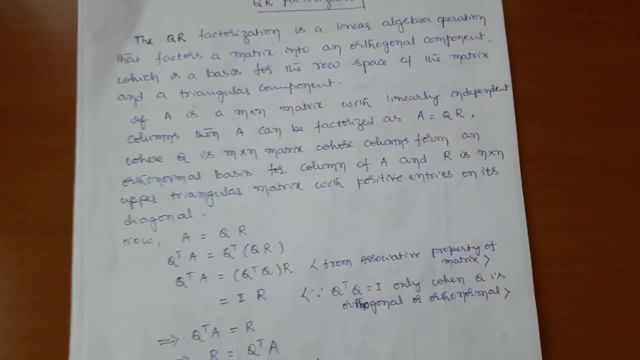 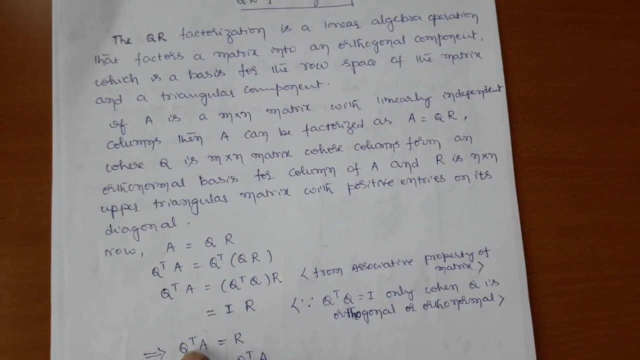 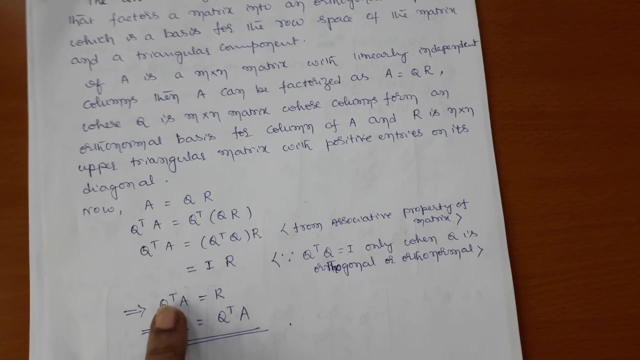 each orthogonal, orthonormal basis vectors are nothing but columns of q. this is a way to form q. once you form q, take, transpose of q into a. but keep in mind a into b is not equal to b into a. commutative property does not hold good under the multiplication. always you take a after q transpose. 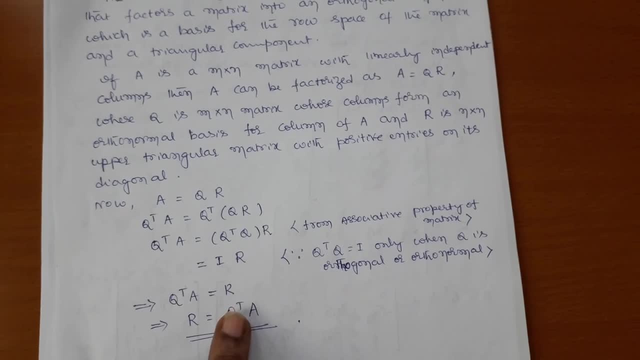 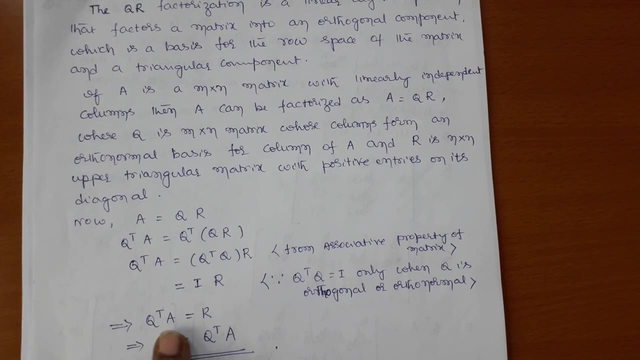 you simplify that you are expecting a, but a is what type of a you are expecting now. a is nothing. but actually, uh, what is a? a? i'm sorry, you q, q, q transpose into a, we get r. r is a upper triangular matrix, but uh, what about positive? 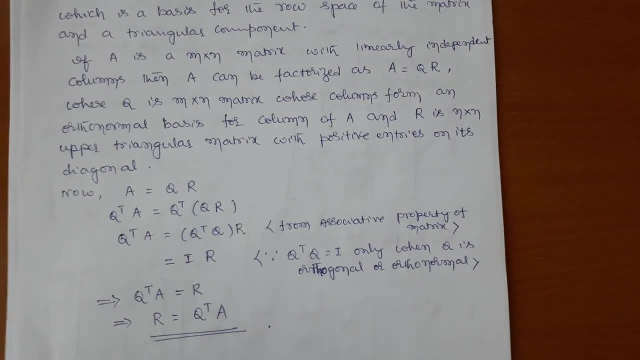 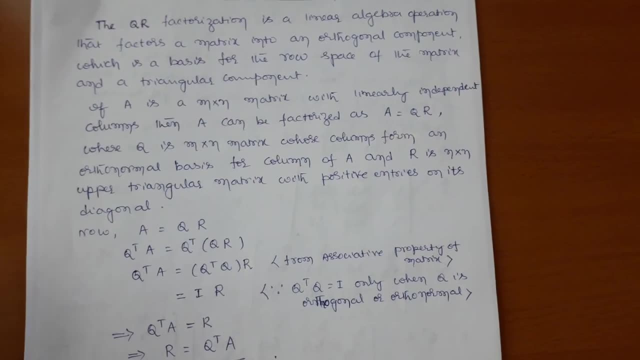 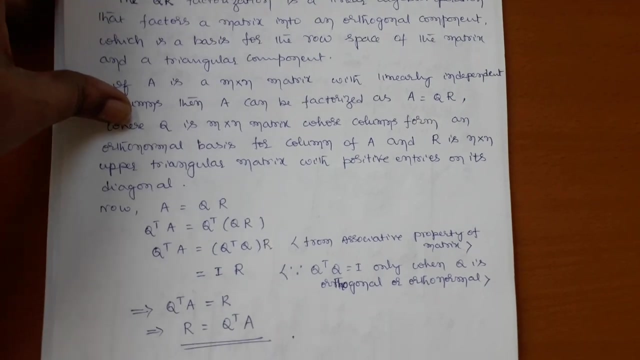 entries on its diagonal. that's the way you are expecting. once you multiply r, q into r, definitely we get a. then only say that what you factorize uh a into qr is nothing but is correct. that is the method for qr factorization. i think everyone is clear for this. i'm moving to the next. 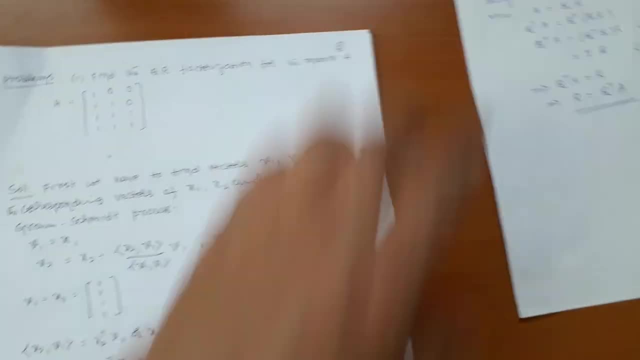 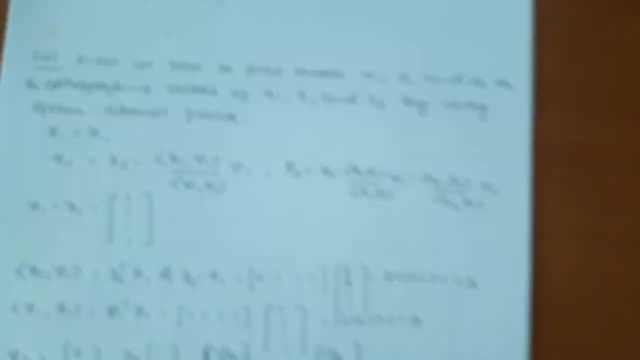 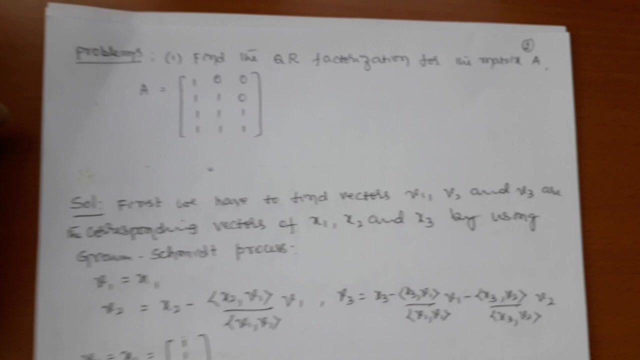 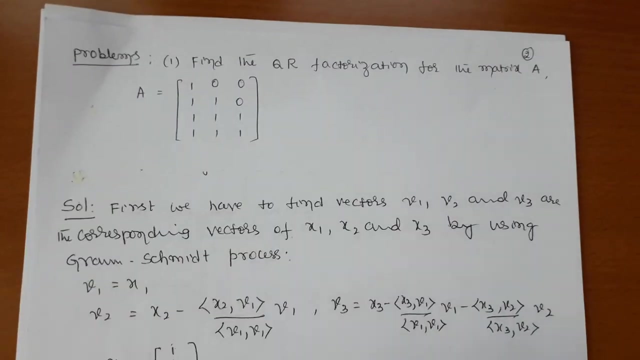 how to solve the problem by using this. okay, yeah, the next step is, uh, we are going to use the next step problems first. problem: yeah, observe cap hosp, sal cap tree in this uh problem, yeah, uh, it's very easy. the problem is, uh, yeah, problem is very easy. suppose you clear grams commuted process, find the qr factorization. for the matrix a they have in the math box. yeah, and then, uh, blade reduction, it is deep. second, also, you depend on what type of r means to allow a and we multiply a to find those are equal a. so solve the problem by adding r into a this time, just Already made. a equation: plus H plus A, d is equal to the both multitude in what says f of r plus B and n minus Q, which is one G цвет in which your vector was same to p, equals i you mean. So we do the r and n plus V and vector used in case ofykp vector and you think if the vector was since드� is being 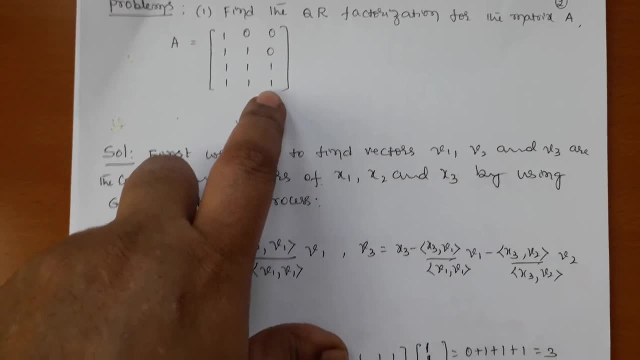 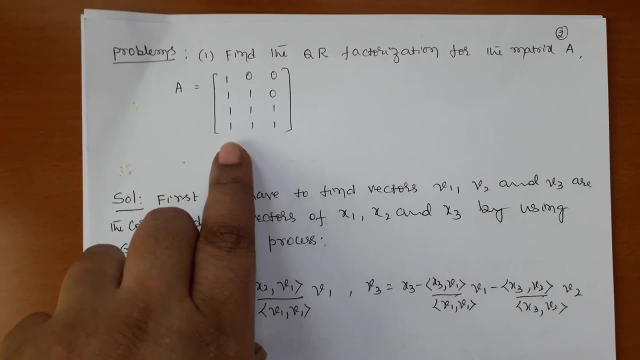 having 1, 1, 1, 1 and 0, 1, 1, 1 and 0, 1, 1, 1. then these observe the how many columns you have: 1, 2, 3. once you write the vector, we get three vectors: v1, v2, v3. observe all three vectors are linearly. 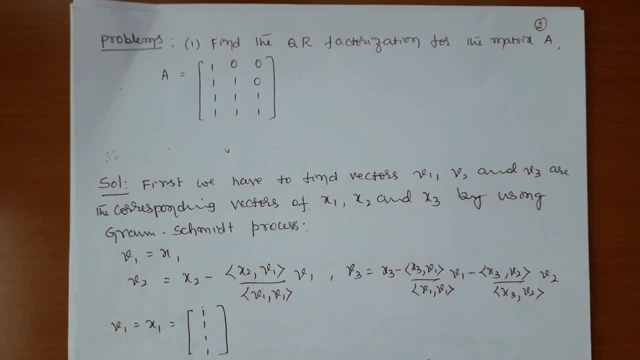 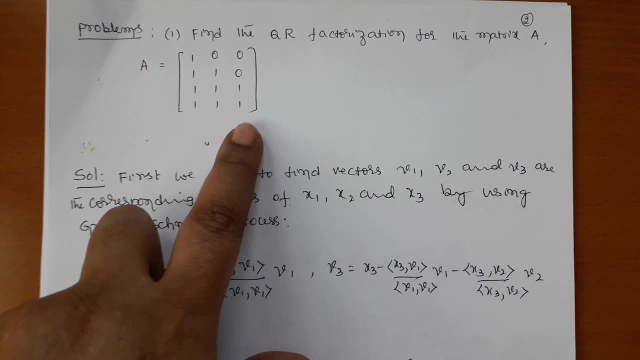 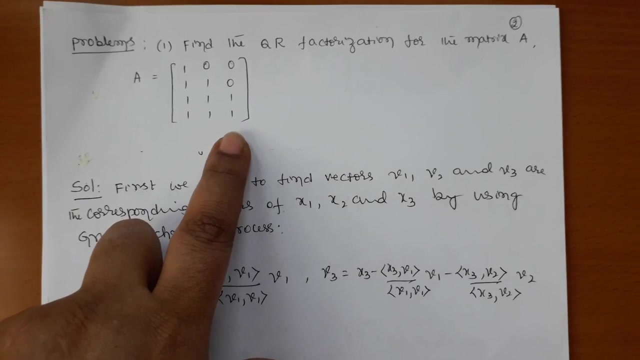 independent. therefore it's possible. i go for qr factorization. if you want to do the qr factorization i told. first you pick the each columns are nothing but v1, v2, v3. first you pick this is v1, this is v2, this is v3. once you pick v1, v2, v3 and sorry, sorry. first you pick these are x1, x2, x3. yes, these 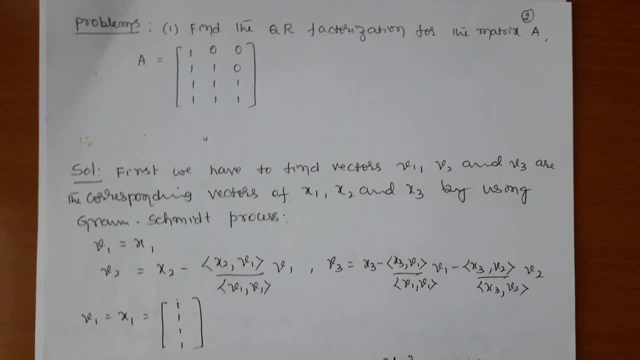 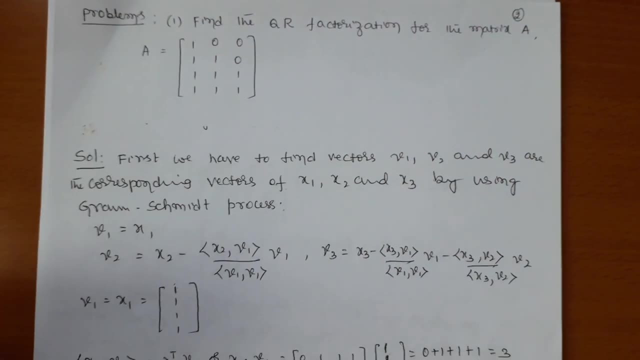 are x1, x2, x3 are the vectors from that, by using grams committed process to find out v1, v2, v3, first, we have to same thing, what we already known, that already. i discussed this problem in grams committed process, even though i'm going to explain. then we get a: what about revision for that? 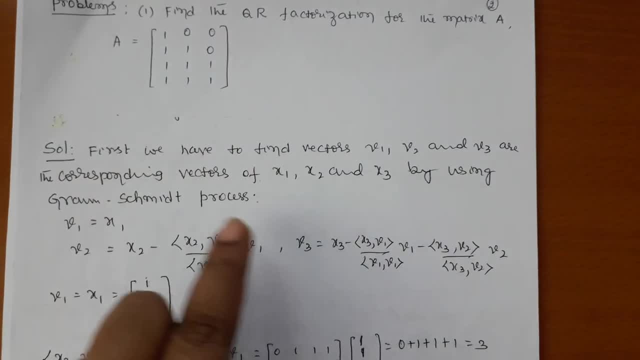 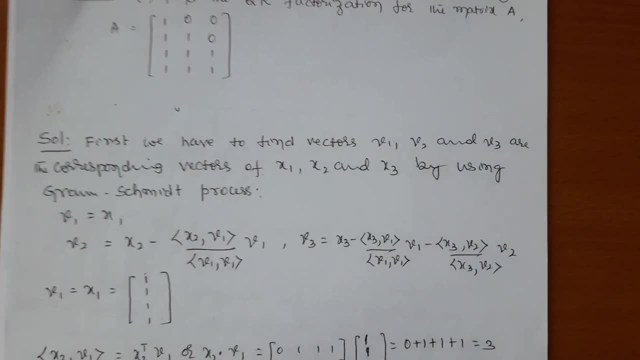 first we have to find vectors. v1, v2, v3 are the corresponding vectors of x1, x2, x3, by using grams committed process. you know what are the formula you already familiar with: v is equal to x1. what is v2, x2 minus inner product of x? 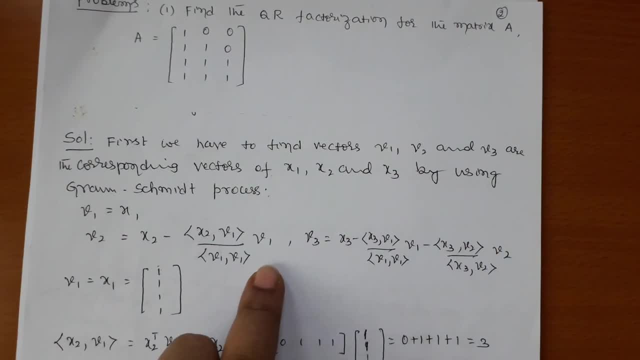 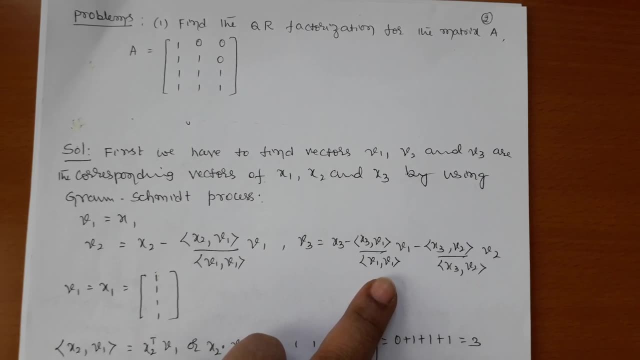 x2 comma v1 divided by inner product of v1, v1 into v1. what's the formula for v3? is x3 minus inner product of x3 comma v1 divided by inner product of v1. v1 minus inner product of x3- v2. 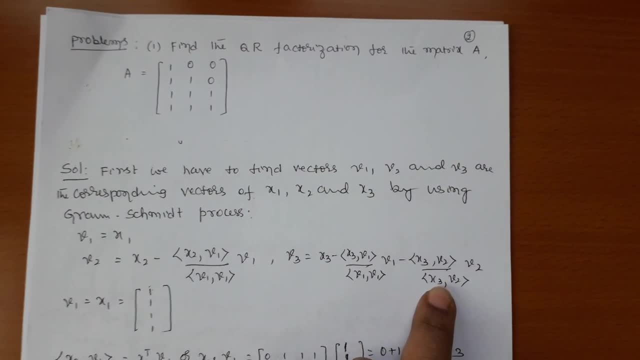 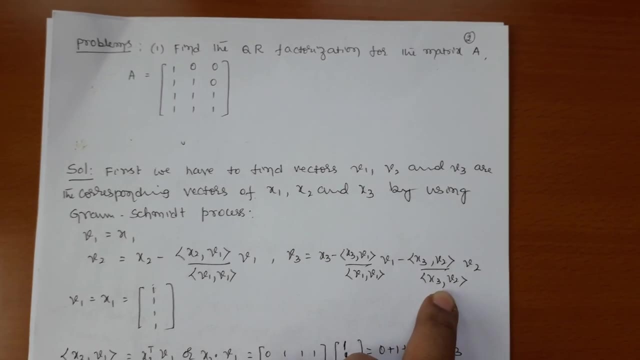 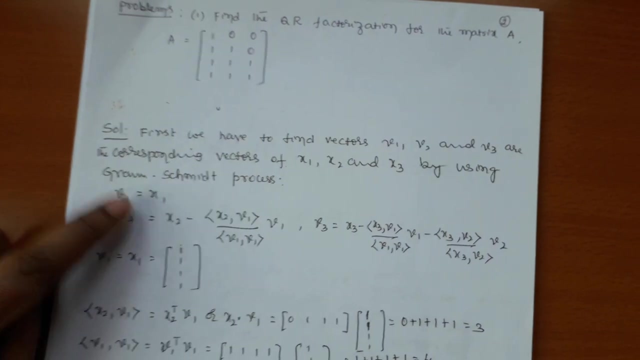 divided by v. actually this is v, v2, v2 is wrong, actually v2. v2 yeah, into v2, actually inner product of v2, comma v2. i'm going to change. this is v2, actually v2. then what is my v1? v1 is nothing. but what actually? x1. 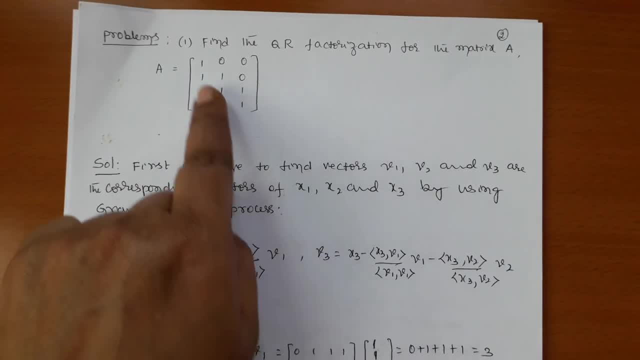 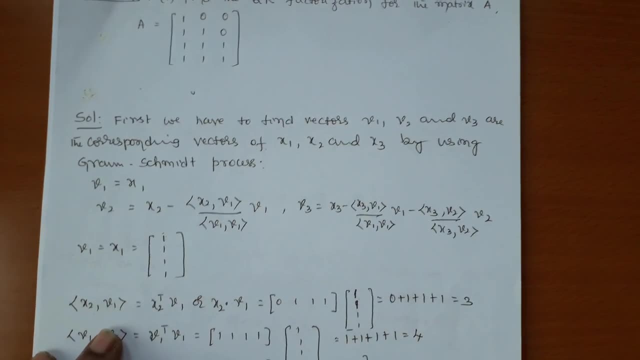 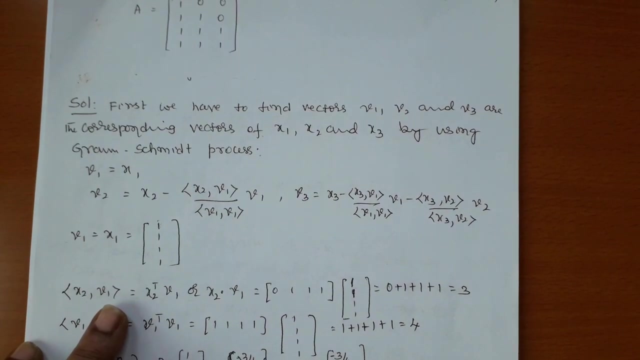 what is x1 here? you already known that in the given what is x1? 1, 1, 1, yeah. next i have to find out what actually v2. while finding v2, v2, inner product of x2, to find out which value first. x2 in a product of v1 is nothing but is a column vector. this can be. 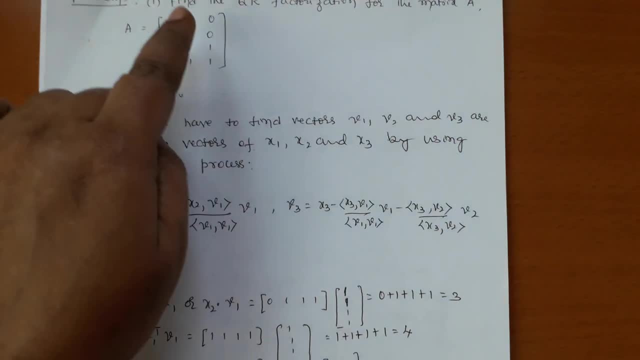 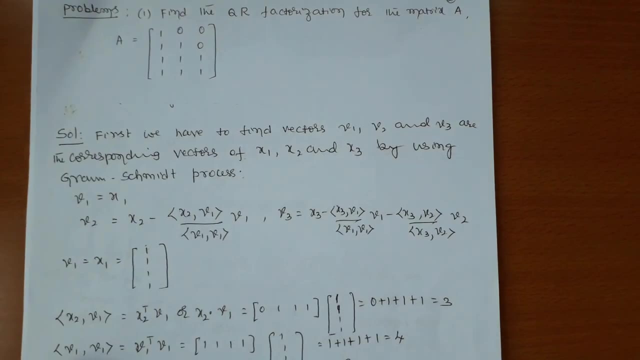 written as x2. transpose into v1: what is x2? they given 0, 1, 1. 1, that's a row into column. this is a vector. multiply that we get 3 and then find out inner product of v1. v1: what is inner product of? 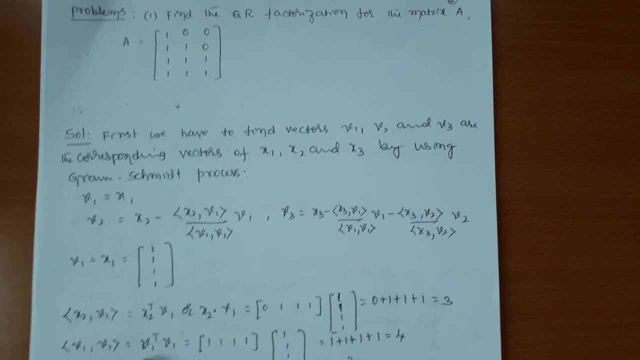 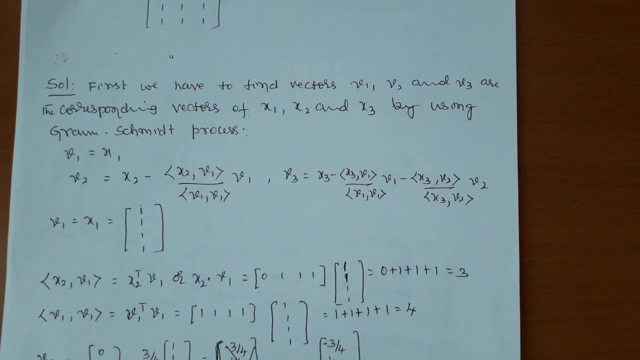 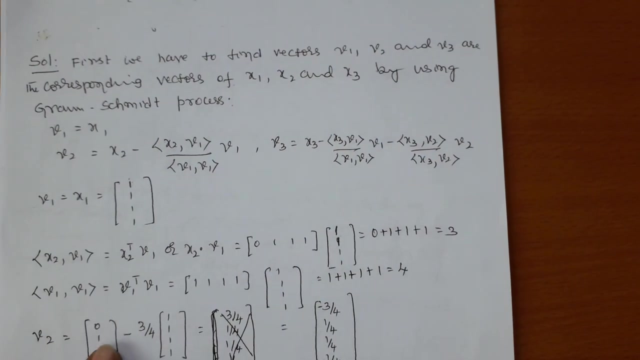 v1, v1. v1 transpose into v1 is 1 square plus 1 square plus 1 square plus 1 square we get 4. yes, then i have to substitute these values where in this one where actually i have to substitute these values, where actually in v2, v2 must be equal to x2. 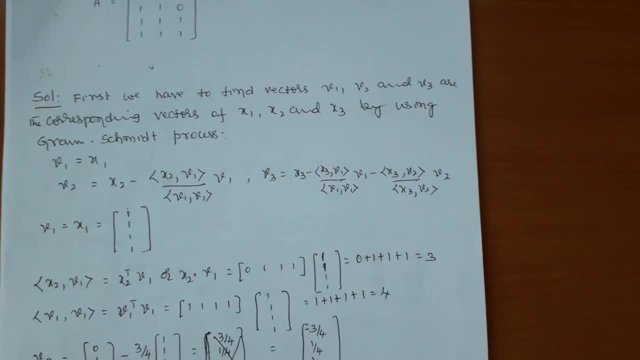 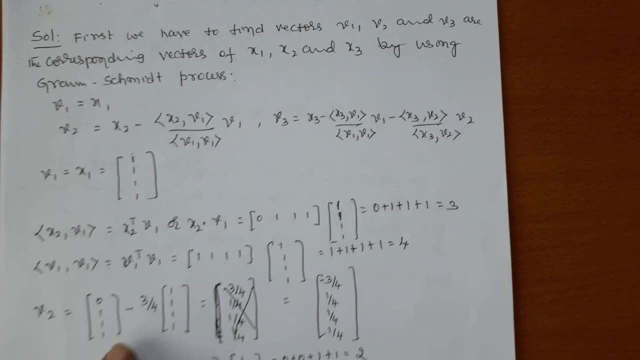 what is my x2 is nothing but 0, 1, 1. i have to substitute 0, 1, 1 minus x2. inner product of x2: v1 is 3 divided by what is the value of inner product of v1. v1 is 4, 3 by 4 into v1. this is v1. 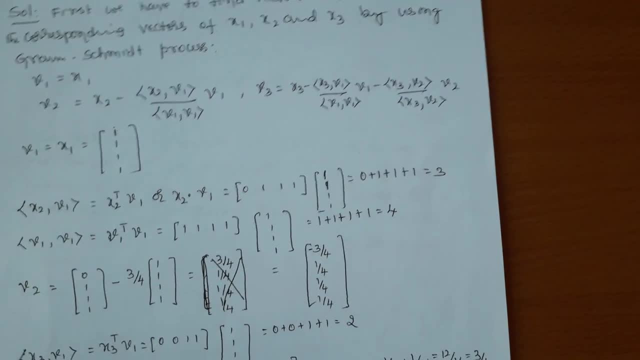 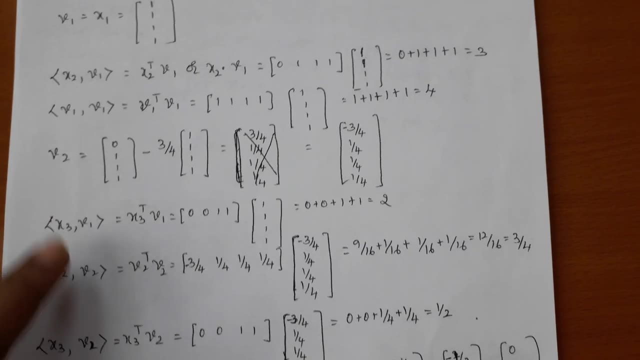 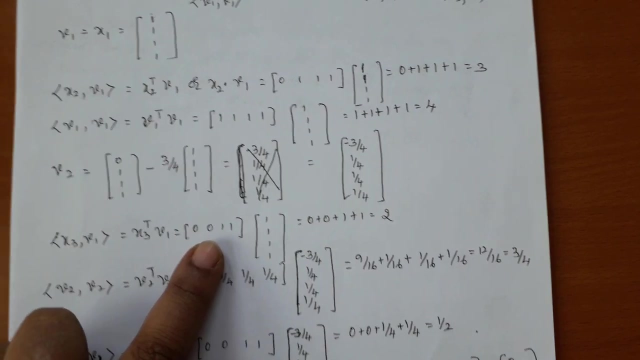 simplify that we get. this is a vector for v2. similarly, i have to find out which way vector v2 vector. if you want to find out v2 vector, what's the thing i want to find out here? first you find out inner product of x3 comma. v1 x3 transpose into v1 x3. is they given already in the? 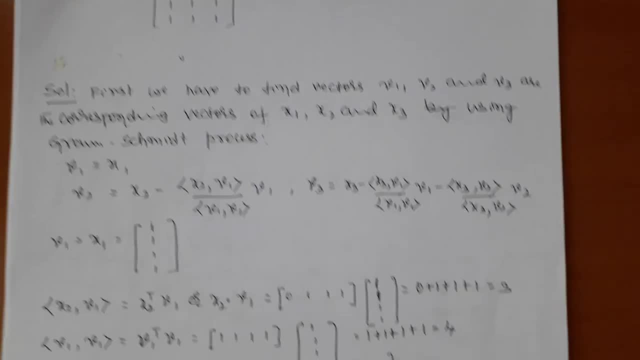 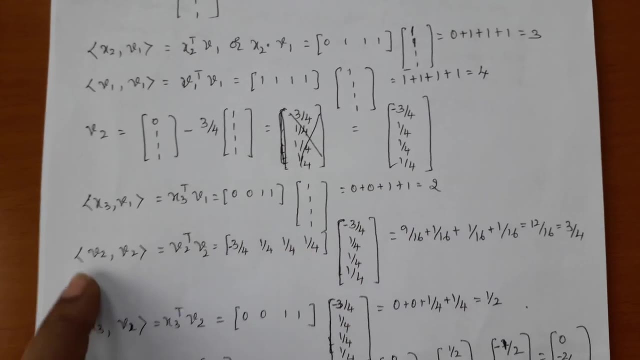 problem. what is they given 0 0 0 1 from that i have to find out 0 0 1 into 1 1. 1 is because v1 simplify that. we get this similarly to calculate inner product of v2 comma. v2 is nothing but v2. 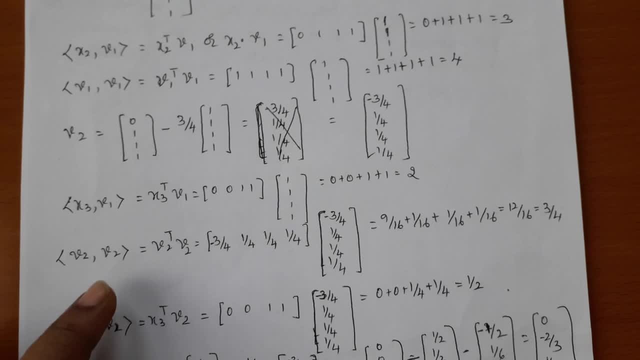 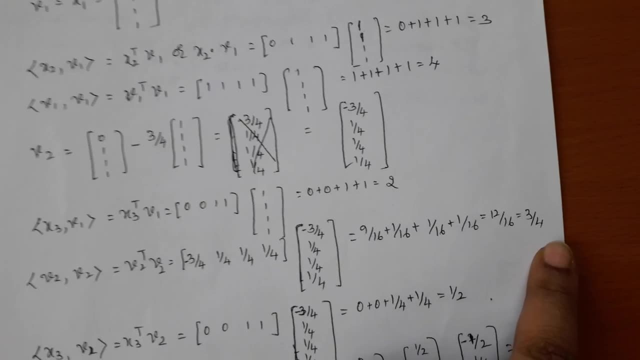 transpose of v2 is nothing but v2. transpose of v2 is nothing but v2. transpose of v2 is nothing. but you multiply, then v2. transpose means you know. you just know what is v2. take in row into column. multiply that after the simplification we get 3 by 4. once we get 3 by 4, what's the next is? 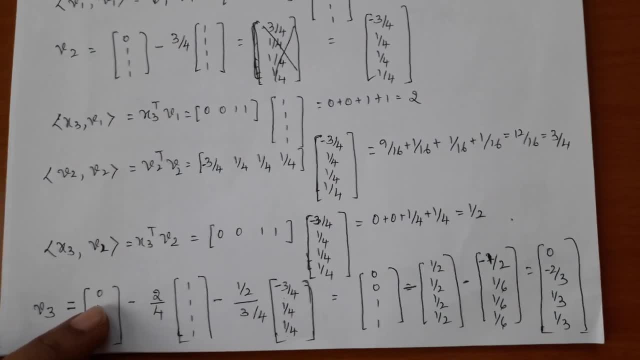 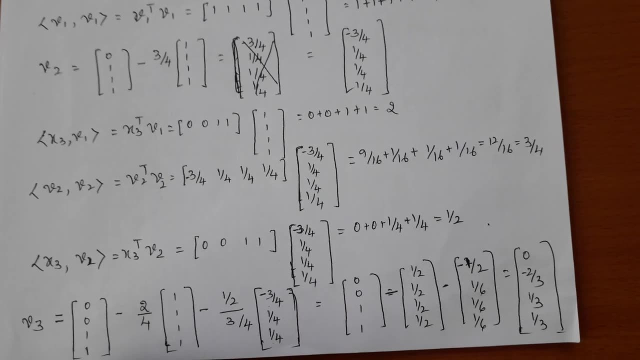 inner product of x3 into v2. x3 into v2 is nothing but x3. transpose v2 again i have to take row x3 row into a column then simplify that. we get 1 by 2. therefore, now i have to substitute these values where in v3 what is v3 and v2? i have to simplify that. we get 1 by 2. therefore, now i have to. 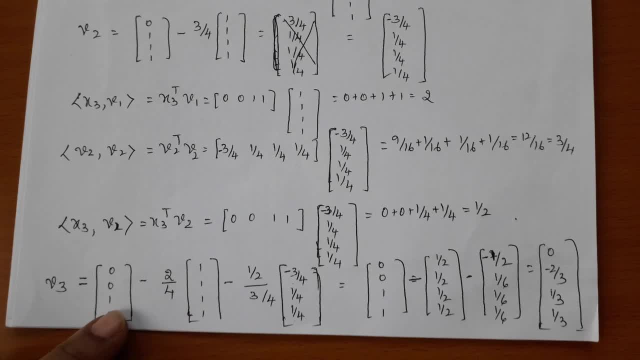 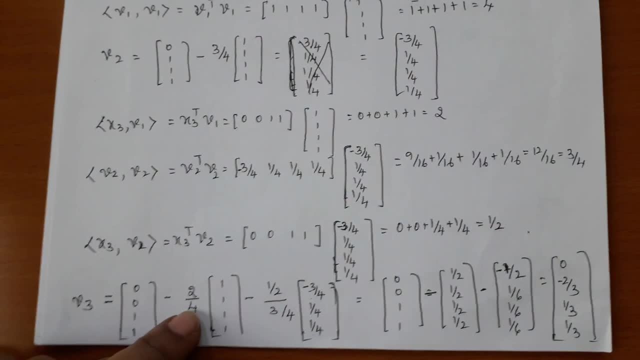 actually v3 is nothing but 0, 0. this is nothing but x3 minus. inner product of x3 comma. v1 is 2. just now we calculated is 2 divided by inner product of v1 comma. v1 is 4, 2 by 4 into v1 minus. 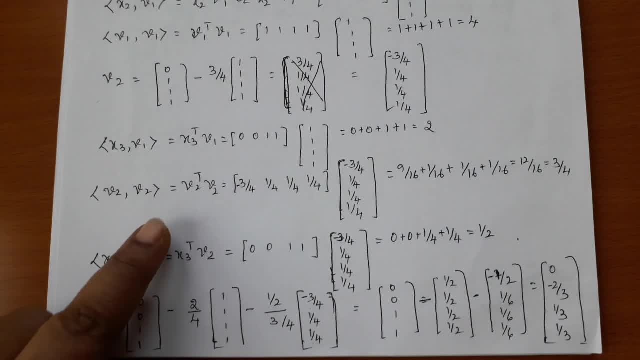 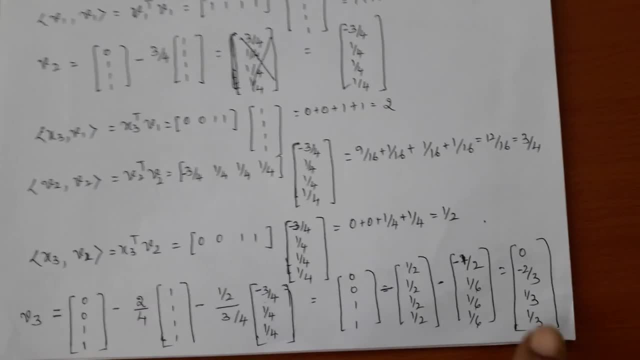 inner product of x3 comma v2 is 1 by 2 divided by inner product of v2 comma, v2 is 3 by 4 into v2, this is v2. okay, then simplify that. finally we get, this is our vector. finally we get, this is our. 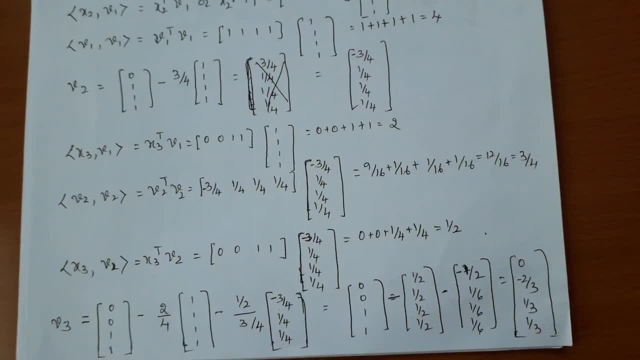 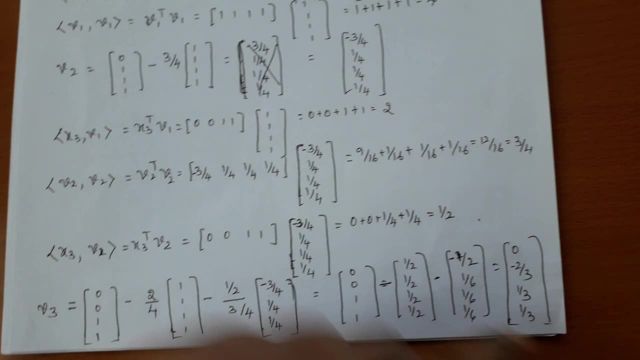 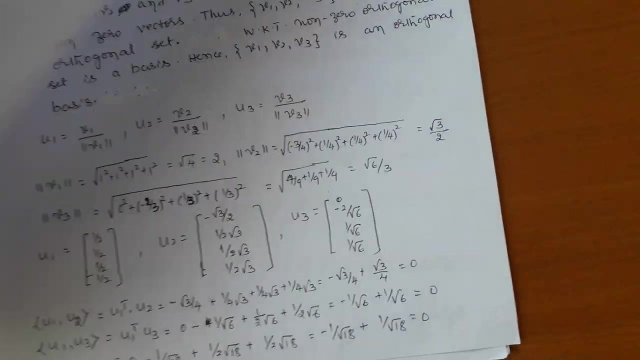 vector. are you clear? this is a vector. a little bit fast, because you know all the steps. that's why i'm i'm explaining little bit fast now, after the simplification, we get this. okay, once we get that, these things, you already know that we're in the grams committment process and then i'm moving to. 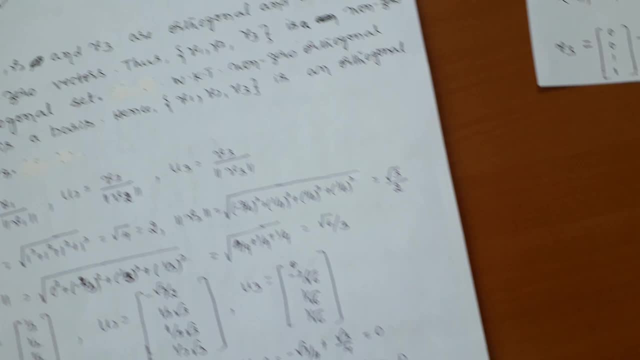 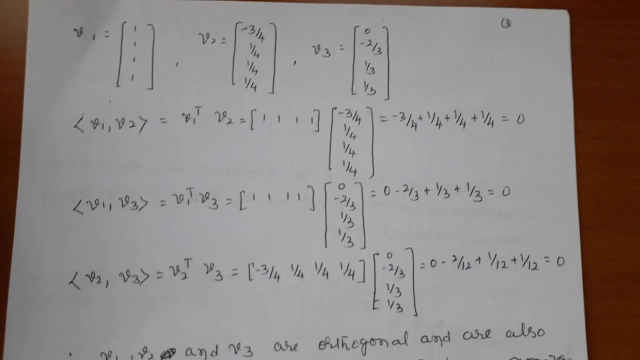 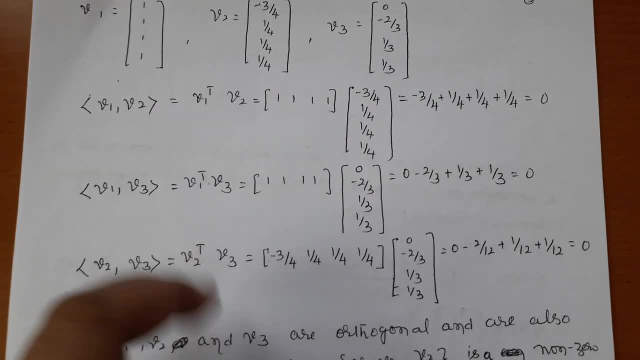 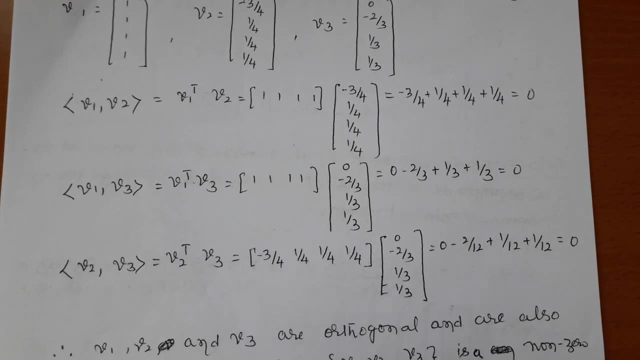 this is v1, v2, v3. i have to verify whether it's orthogonal or not. how to verify? take inner product of v1 comma v2, calculate inner product of v1 comma v3 and then inner product of v2 comma v3. it's nothing but v2 transpose v2, v1 transpose v3 and then v2 transpose v3. you know how to. 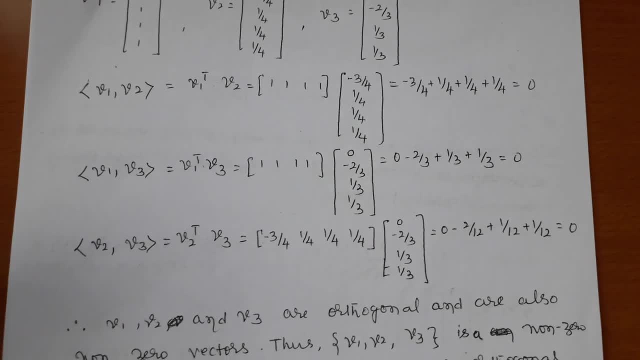 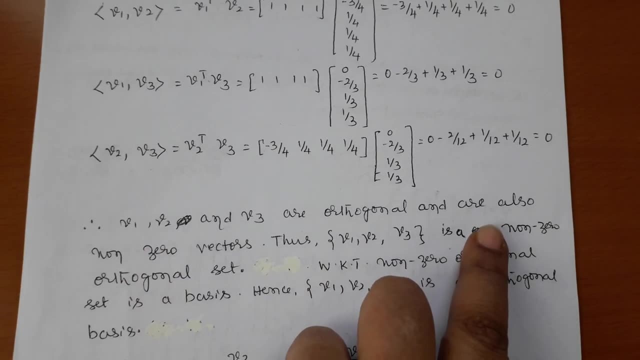 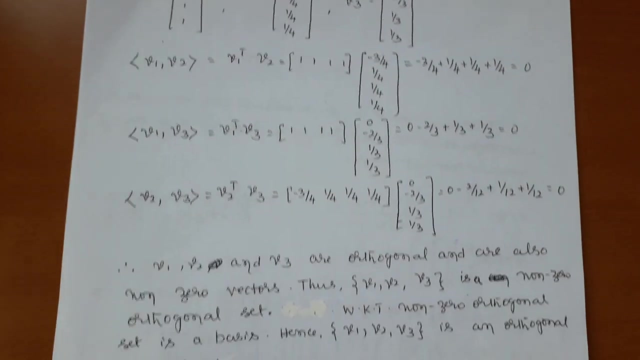 calculate this part already explained in grams committed process, then all are zero. then we say that therefore v1, v2, v3 are what actually orthogonal set, orthogonal and also non-zero vectors, because v1, v2, v3 are clearly non-zero vectors. yeah, and the next therefore thus v1, v2. 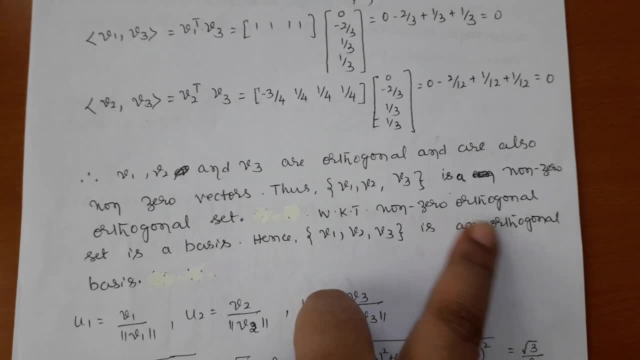 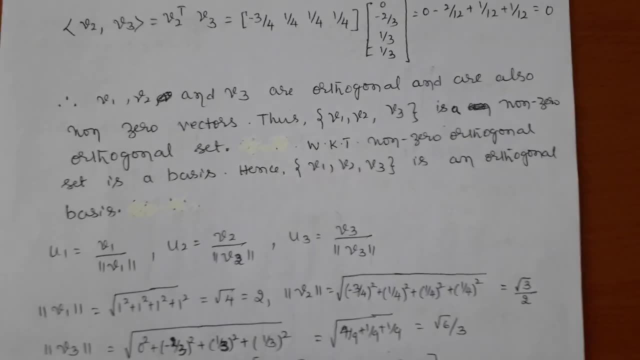 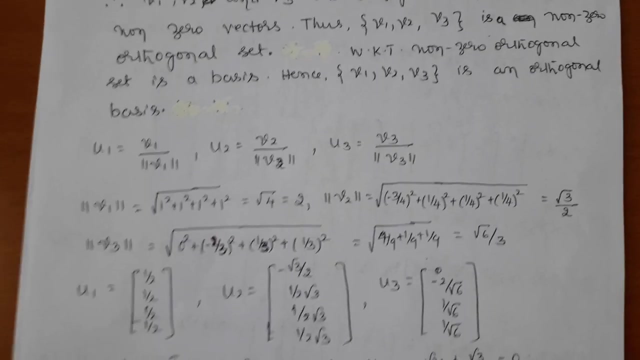 v3 is a non-zero orthogonal set. we know that non-zero orthogonal set is a basis, hence v1, v2, v3 is a orthogonal basis, but q is nothing but the columns of a for the orthonormal basis of a, columns of a. next try to find forthongonal orthonormal. 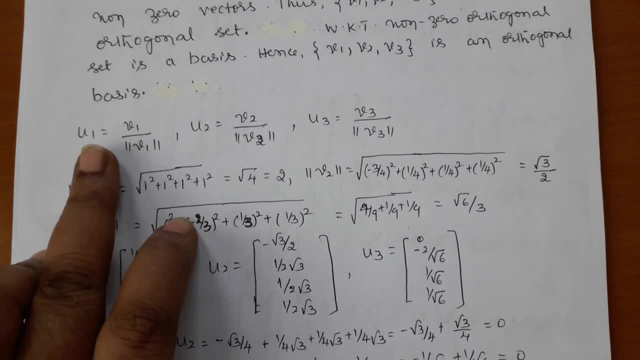 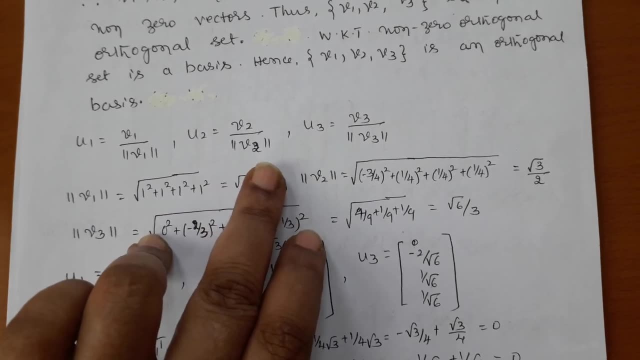 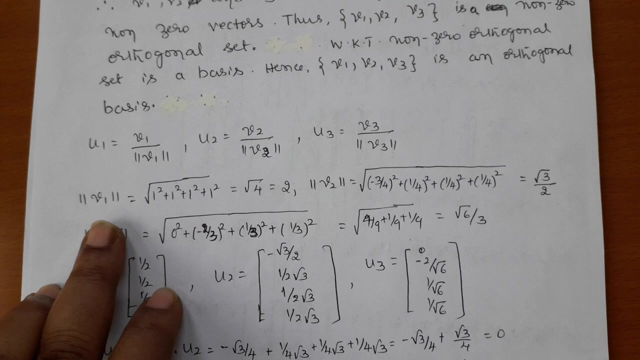 set. how to find out artтаки set, we already discuss in the previous slide video. u1, v1, v1 divided by norm of v1, u2 is nothing but v2 divided by norm of v2, and then u3 is nothing but v3 divided by norm of v3. you know how to find out? what about that norm of v1 norm? 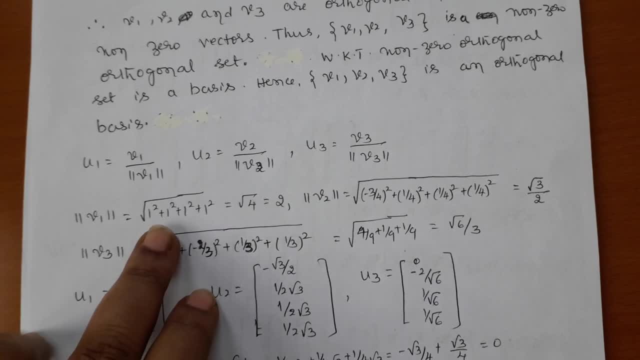 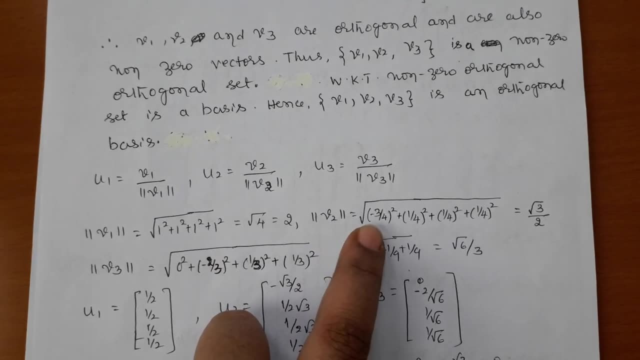 of v2 and norm of v3. norm of v1 is nothing but square root of straight square. right from the beginning, this thing is, you know how normal set of vos another. each of the value v1 value, 1 square plus 1 square plus 1 square, we get 2. norm of v2 means square of. 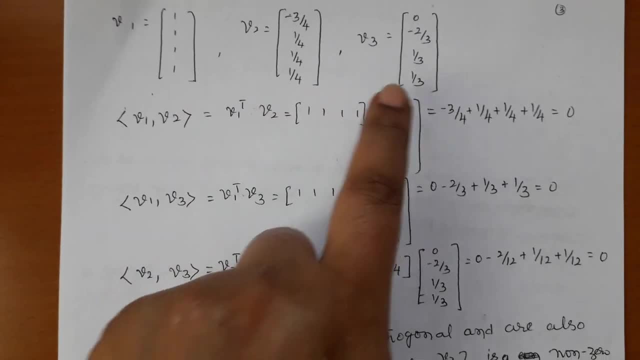 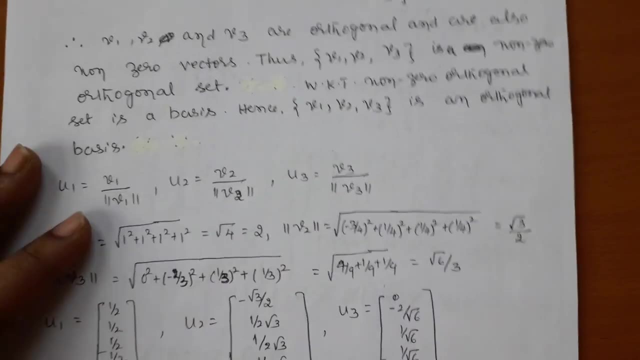 the each of v2 value. you already known that this is v2. similarly, i have to take square of each of the value of v3 is nothing but norm of v3, the square root of that. simplify that we get. this is a value we get. yes, this is a value we get. once we get this value, substitute in u1- i have to divide. 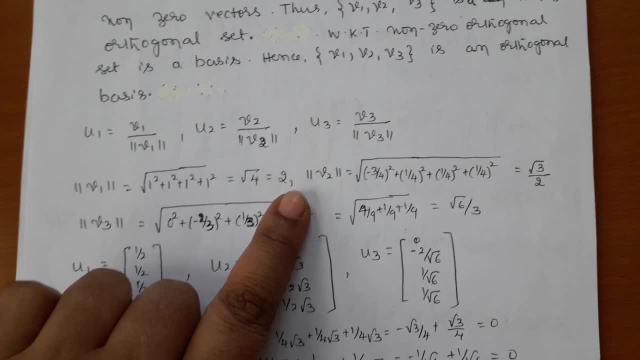 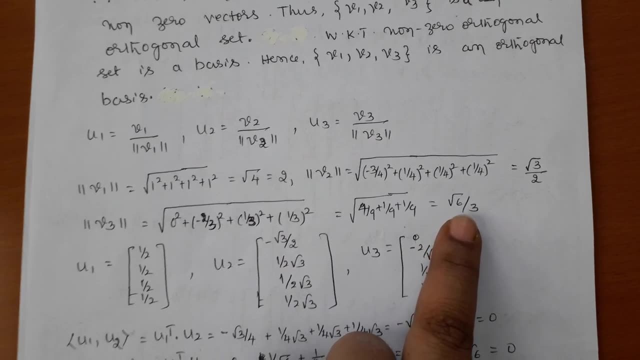 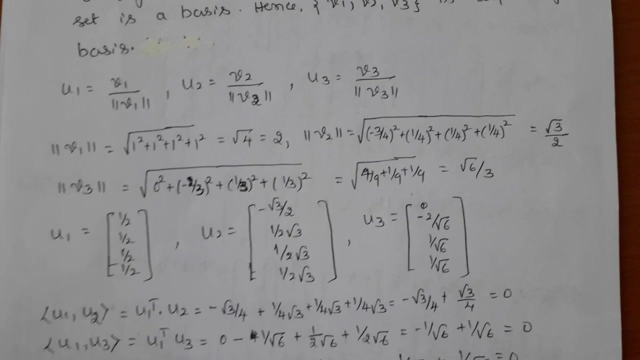 v1 by 1, by divide the v1 by 2, divide v2 by root, 3 by 2, divide v3 is nothing but root. 6 by 3, we get finally. these are the vectors for u1, u2, u3. once we get u1, u2, u3, then i have to find out: is a? 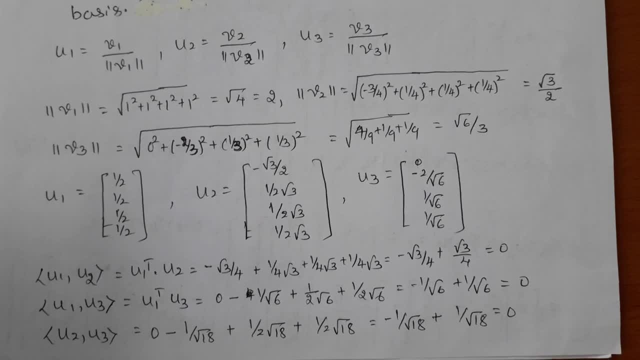 orthonormal set. orthonormal set means: inner product of ui uj is equal to 0, for i is equal to j. inner product of ui uj is equal to 0, for i is equal to j. inner product of ui uj is equal to 0, for i is equal to j. 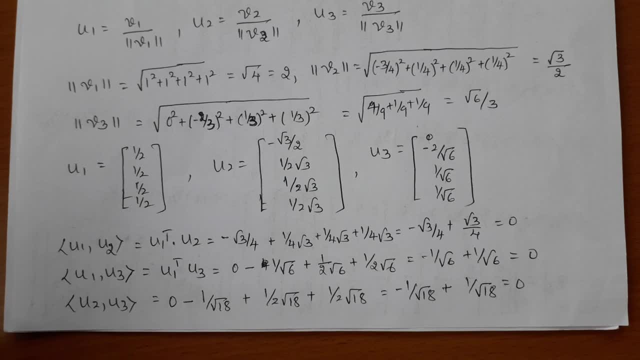 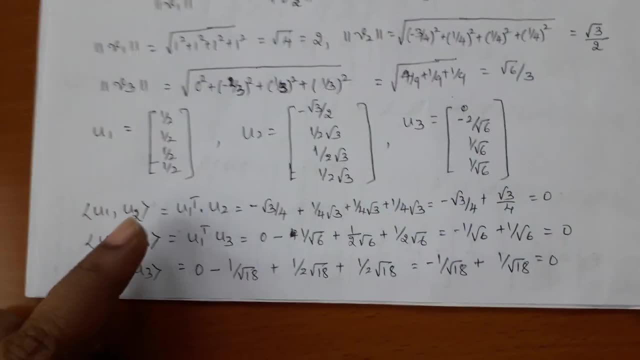 of ui. uj is now equal to now, not equal to 1. i is equal to j then then we say that is a orthonormal set. yeah, similarly, i have to find out what's inner product of u1- u2 is we get 0. inner product of u1. 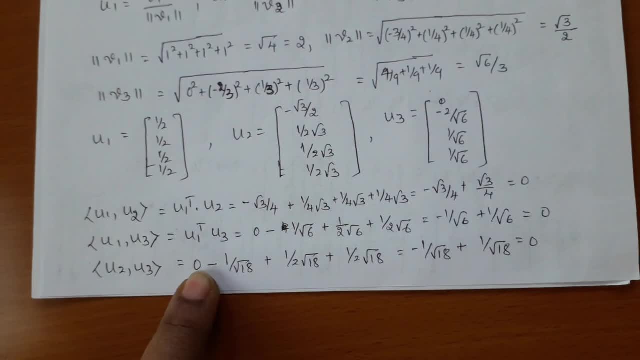 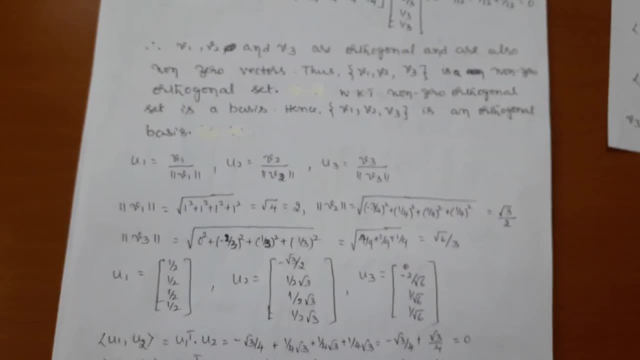 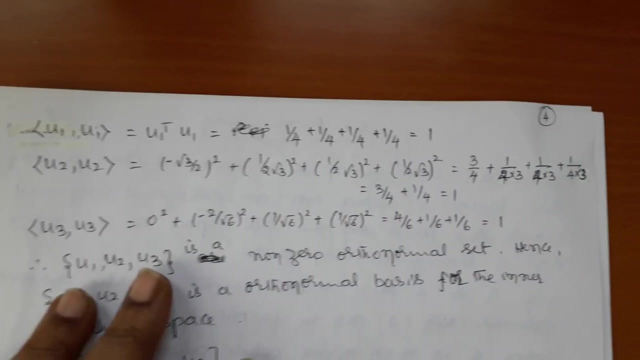 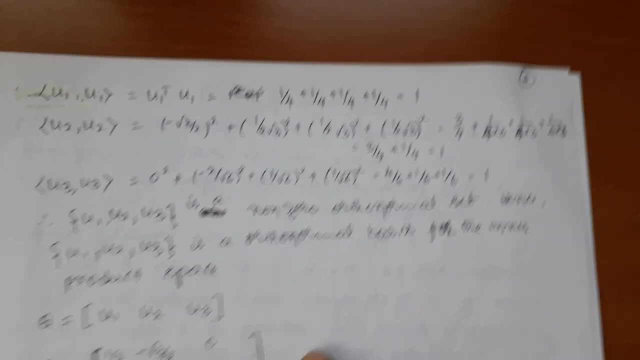 u3 also 0. inner product of u2- u3 also, we get 0. this shows that these are orthonormal, but i want to verify: is a orthonormal means? further, i calculate the values of what actually u1 inner product of u1 comma u1. what's inner product of u1 comma u1 inner product. 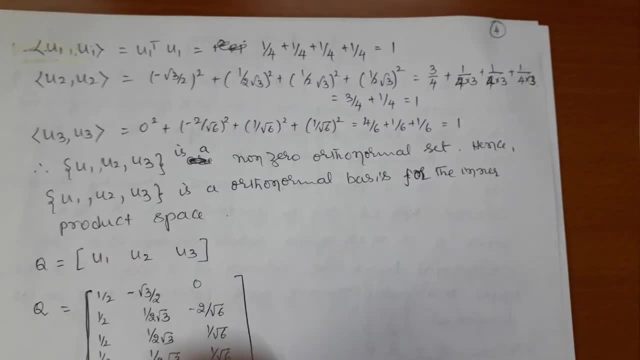 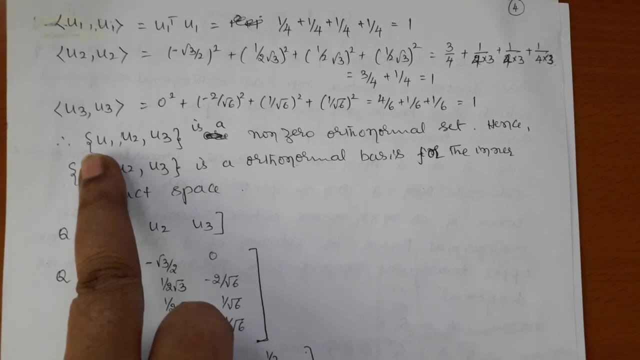 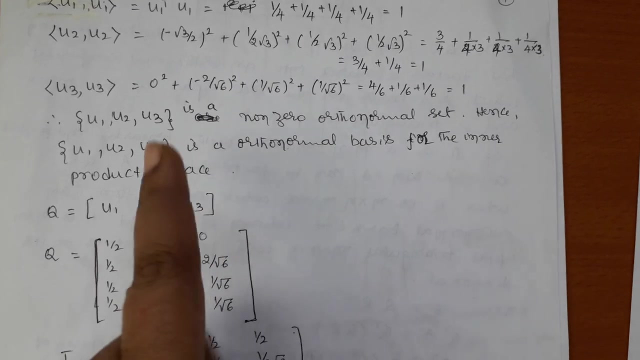 of u1 comma u1 is nothing but 1. here we get inner product of u2 comma u2. we also get 1 after the simplification, similarly inner product of u2 comma u3. what we get is 1. this shows that u1, u2, u3 is a. 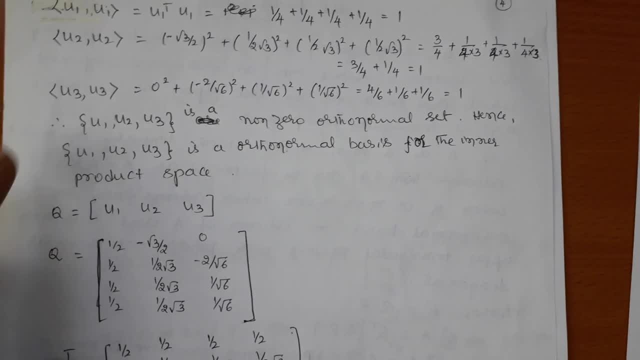 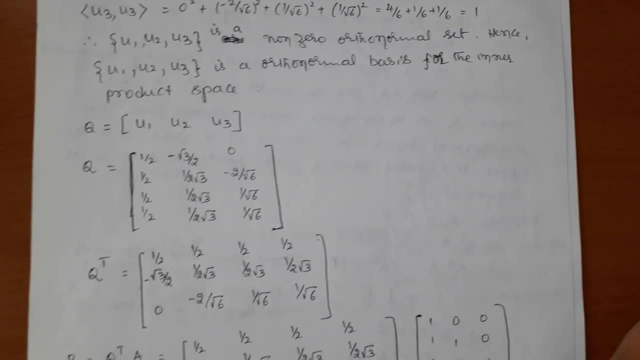 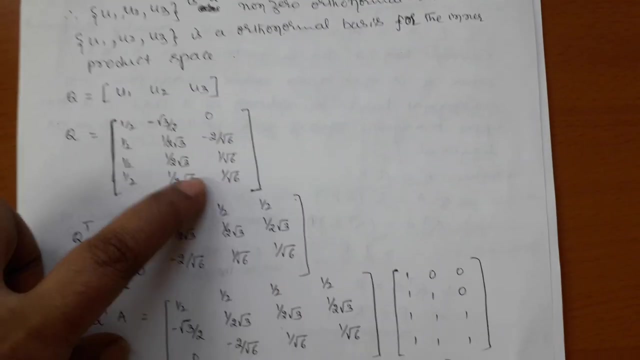 inner product space. now we have to write what is my q. u1 is the first column of q, because these are orthonormal basis for a. we have taken columns of a. you find out the orthonormal basis, the form a, q is a columns of orthonormal basis of columns of a. u1, u2, u3, substitute once we get to take a. 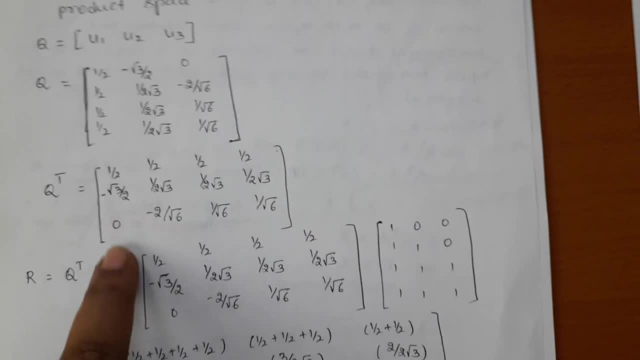 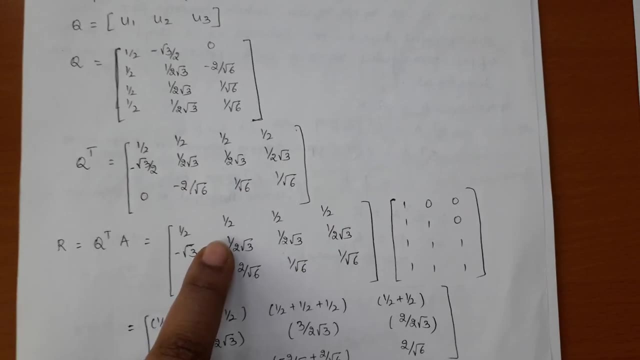 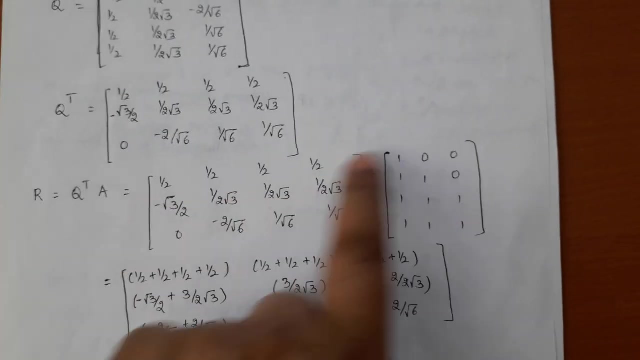 transpose. transpose means what? row into column? yeah, row into column. i return now see: row into column. then what is our q transpose into a right q transpose? you have a, a value they given in the problem is a substitute, and multiply row into column. you have to multiply row into column. multiply. now, this is a first element. you know how. 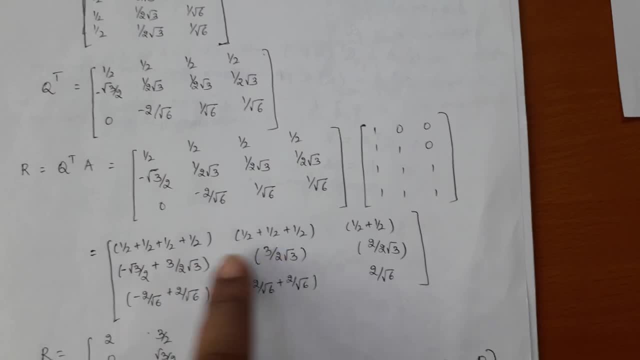 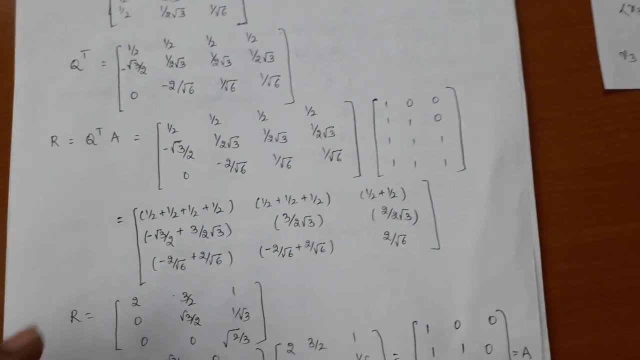 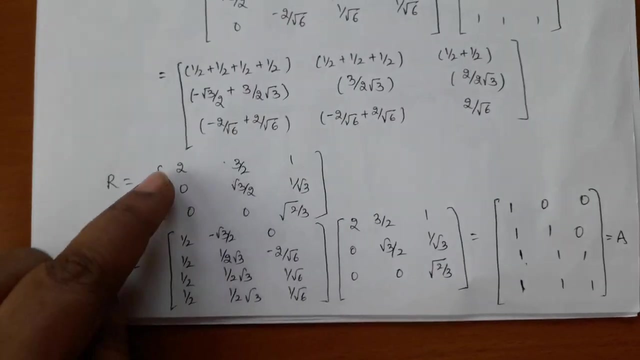 to multiply two matrices. you multiply this written, each and every value. multiply row into column three column. we get three values. second row with three columns. third row with three columns. you get again three. class three matrix. after the simplification, we get r. r is a upper triangular matrix, diagonal. 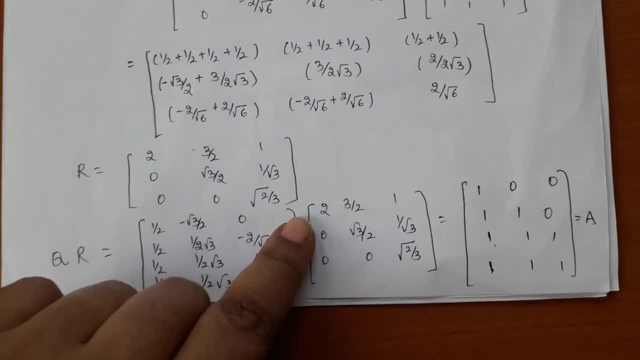 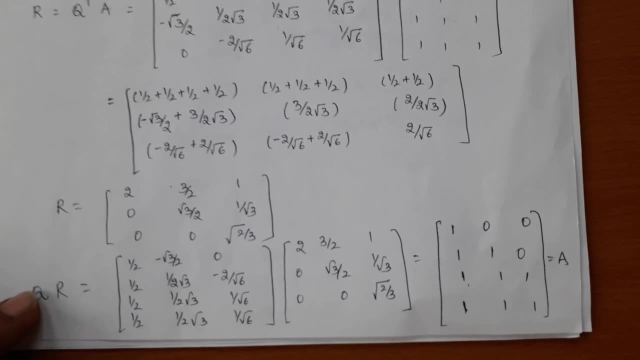 entries must must be a positive, not for non diagonal. diagonal entries must be positive and upper triangular satisfies. and before going to wind up this problem, i want to know whether i convert the factors q and r is correct or not. i have to multiply q and r, then this is students. 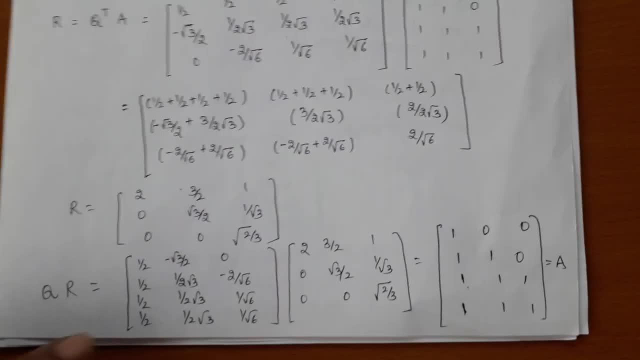 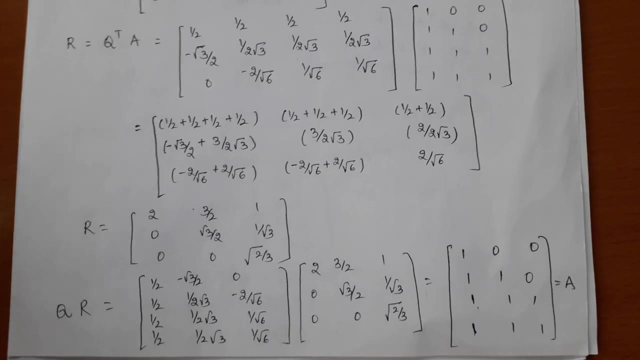 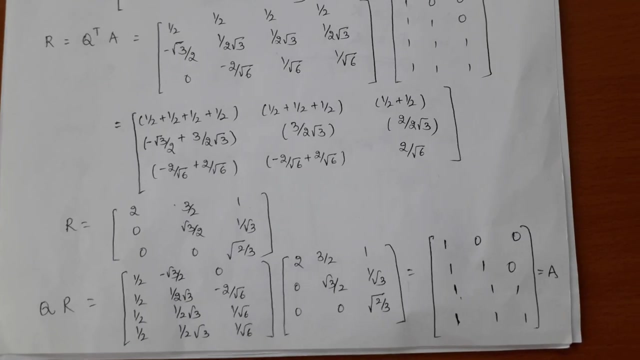 they're doing mistake, even though don't get it. after multiply q and r, they simply writing a. but keep in mind everyone. they are very sharp compared to you faculties. they already knows what they expecting q, what they expecting r. expecting more than that. we are expecting q r, r must be a unique. suppose you did correctly. 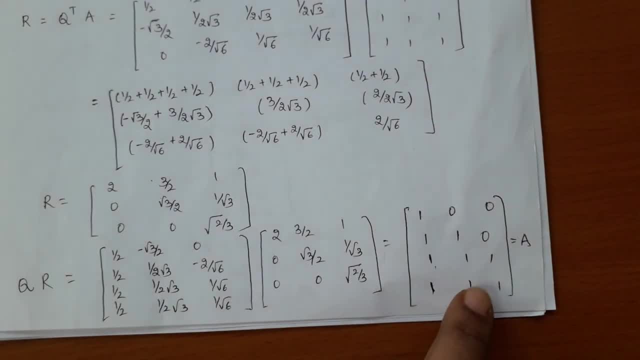 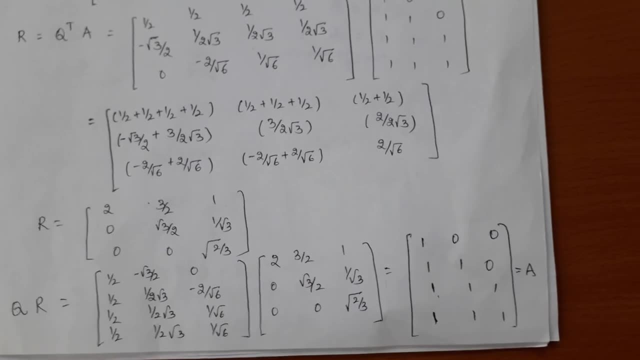 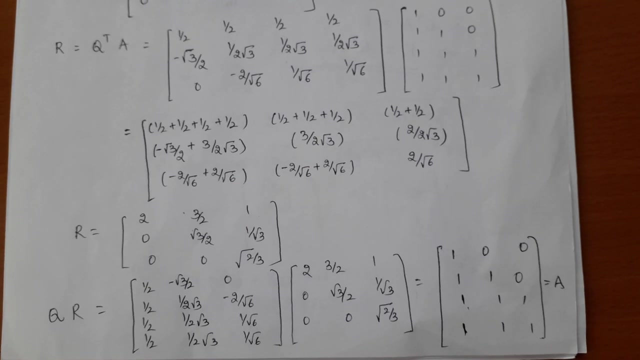 okay, once you multiply that row into column. definitely after i multiplied, only verified, only i return this. i'm not written directly. okay, i did calculation in separate graph book and then i substitute the value: this is vga. then i confidently say that what i done, a solution. 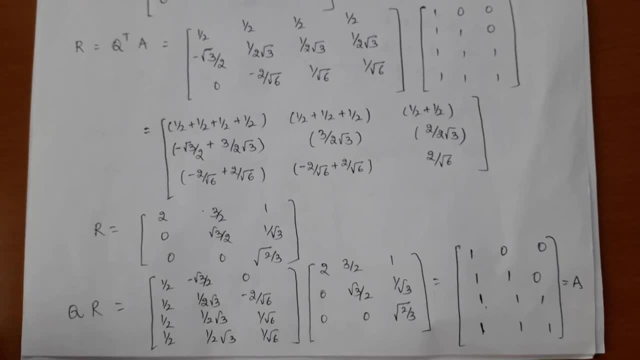